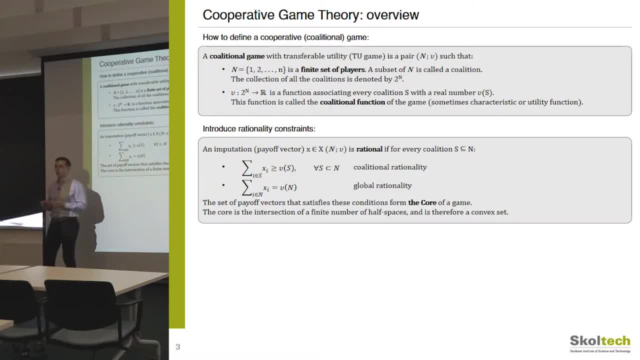 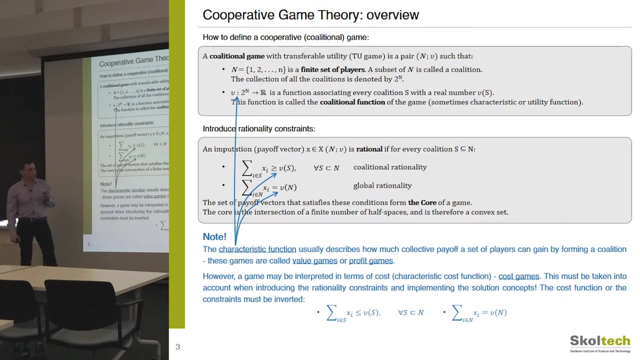 concepts work for simple examples. you remember the gloves examples, the dinner example and everything was fine. So at this moment we should discuss some issues about this concept. and first note you should be careful when using these conditions because they differ for different games and this depends on what you are allocating: the cost or 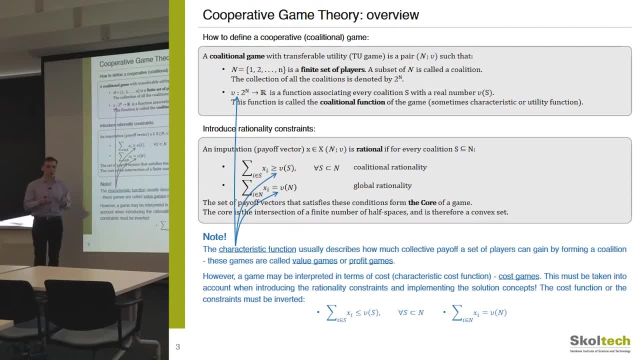 some benefits and if you allocate some benefits, some gain that the players get together. these kind of games are called value games or profit games, and this means that players together should get some more than separately. and there are some games in terms of cost games and for these games you should reverse this condition or invert the characteristic function and 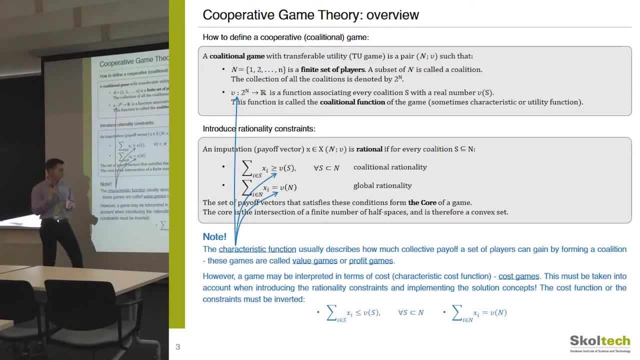 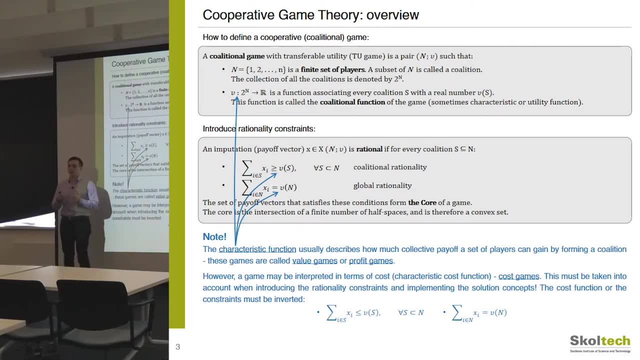 you may. also, you may often check your logic. for example, in case of allocating costs, you should check that for each coalition, the value that they're allocated is less than their own value, because you're allocating costs and everyone wants to decrease its own costs. so this is the first note. 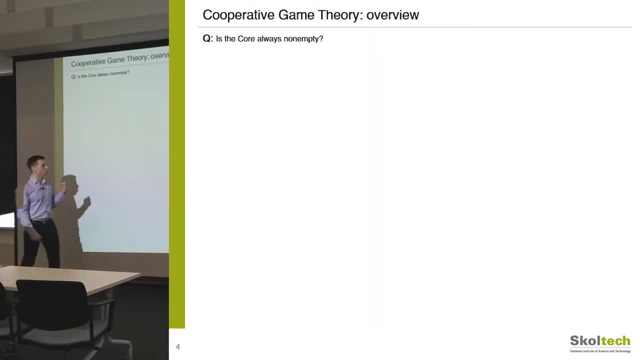 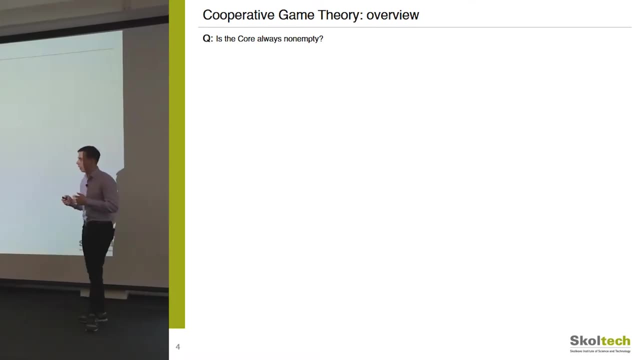 and the second question that we need to ask: is the core of the game always non-empty? the core is defined by this set of rational constraints and, unfortunately, the answer is no. There is no guarantee that the core of a game would be non-empty and therefore we need to discuss. 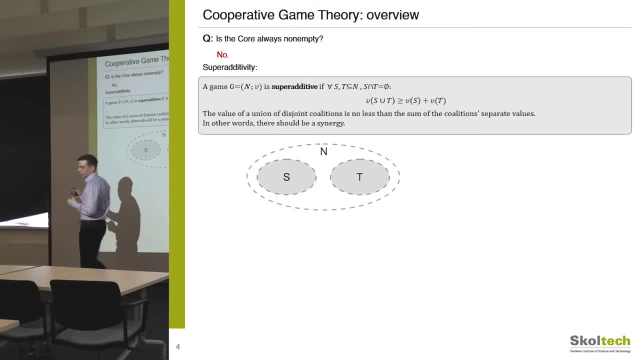 a few more concepts, and the first concept is called super additivity. You may consider two sets of players, s and t, two coalitions- and please notice that they do not cross, so they do not have any players in common- completely independent coalitions- s and t. and super additivity means that it says that 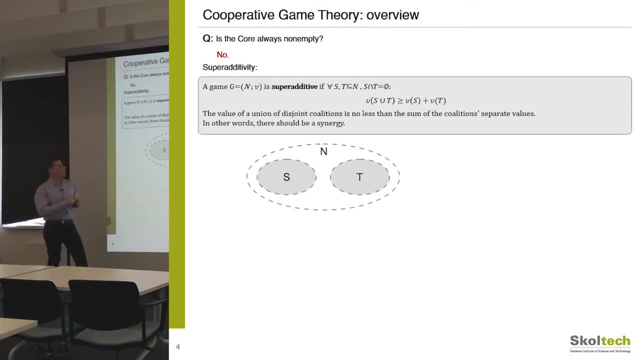 the value that this union, this coalition, is going to have is going to be less than the value of the game. The value that this coalition s plus t gets is greater or equal to the values that players get separately, and, in other words, super additivity means that incorporation should be some level. 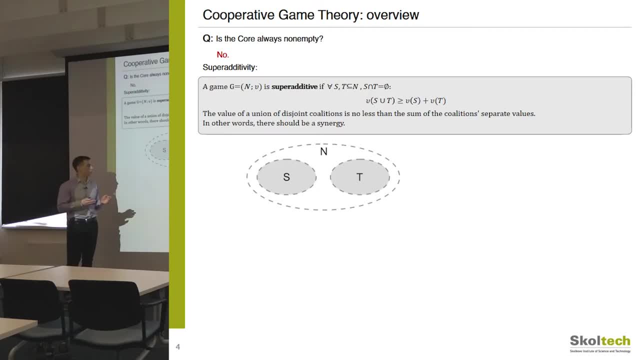 of synergy, it is not simply a sum of their gains. but this is not strong enough condition, and therefore we introduce here the second definition that is called convexity, and the convex game says that the value that coalition s plus t gets should be greater than the value of coalition s plus the. 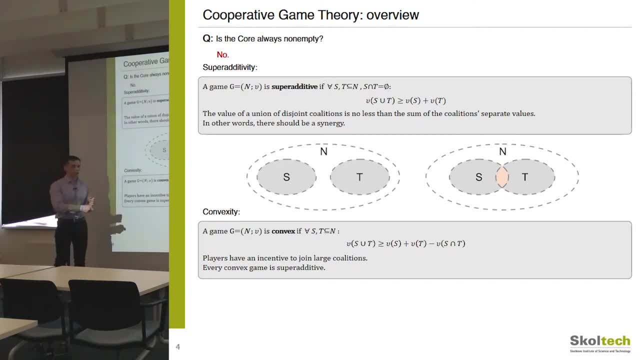 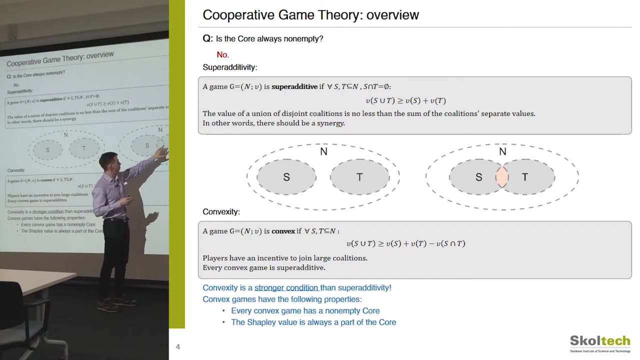 value of coalition t and minus the value of their intersection, this is uh, this is a more strict, a stronger condition, that's superactivity, and it means that there should be some significant level of synergy. so s plus t is much greater than s plus t minus their intersection. and if we find a game, 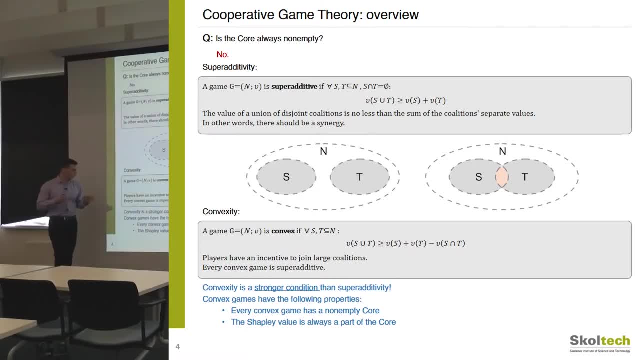 that satisfies convexity, then everything is good, because this means that this game has a non-empty core and, moreover, it is proven that the allocation concept as a shepley value, the solution will be in the core. so you you probably get the idea that once we formulate a certain game, a certain 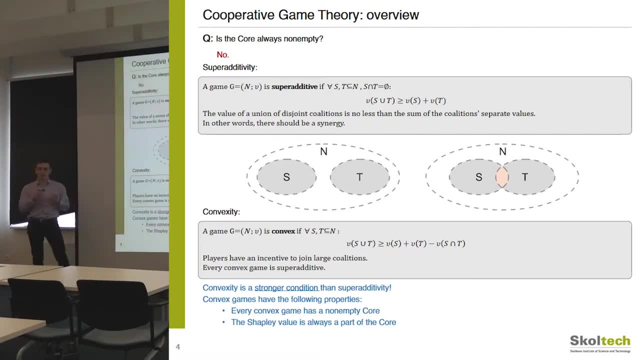 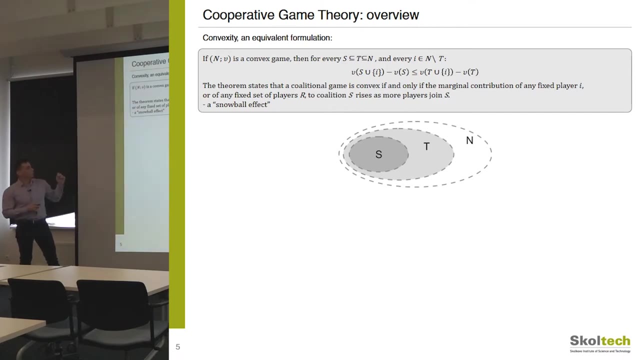 collational game. we need to understand is it a convex game, is it a super relativity game or not, and this would be helpful for the analysis. and let's go further and introduce an equivalent formulation of convexity that i like more than the previous one, and in this case, to introduce it, imagine that set s and t they 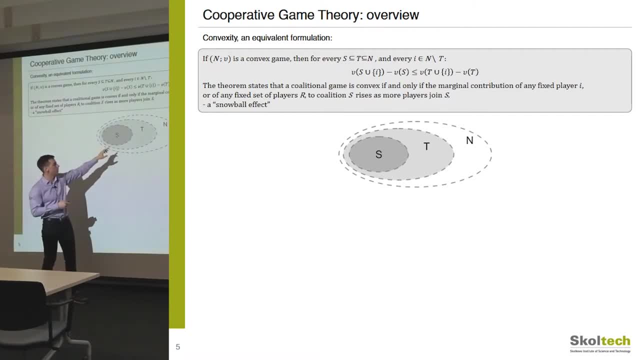 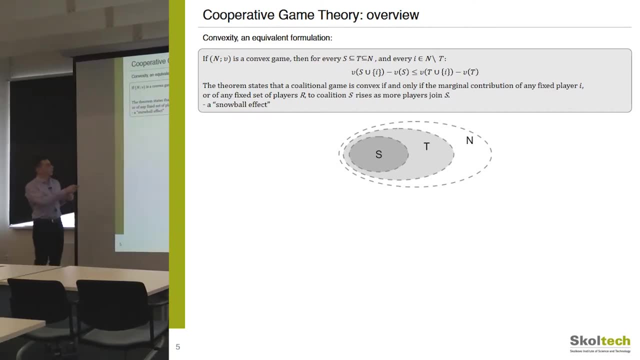 it happens that s fully belongs to t, so it is s less than t and set of players s fully belongs to t and in this case superactivity formulation says that the marginal contribution of player i to collision s should be less or equal to contribution of the same player i to collision t. 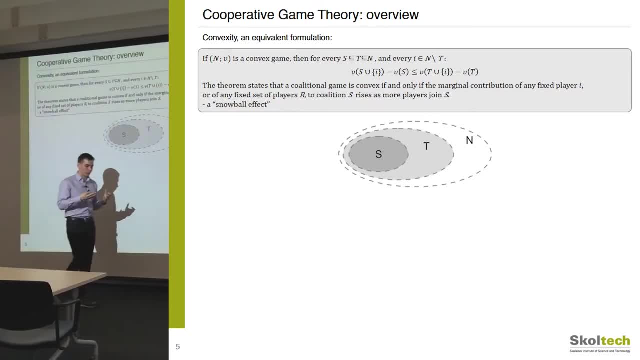 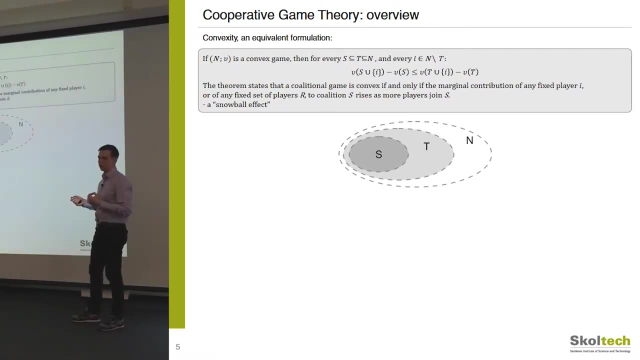 so this formulation tells you that it should be more beneficial for players to join the larger collisions, and this effect is some co, some sometimes called a snowball effect. marginal contributions to collisions with more players brings more benefits, not less, not less, and this is the condition by by what you get. 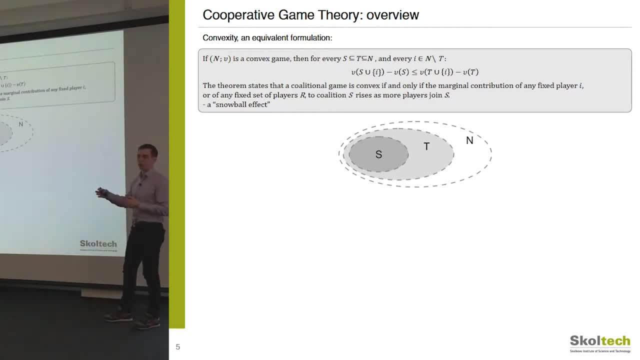 can check every game, every characteristic function that you got. you may program this condition several times, as many as many players you have, as many scenarios you have, and identify easier game convex or not. if it's convex, you shouldn't worry, and all the concepts as the Shapley value will work. 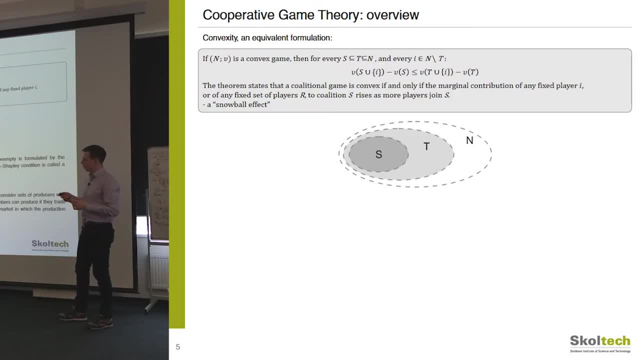 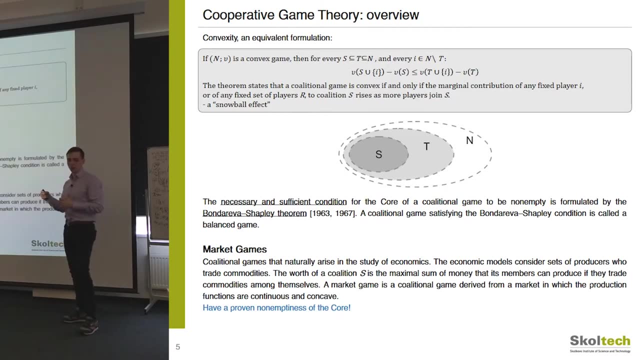 okay, if you wonder about the necessary and sufficient condition for the non empty core, there is a bond- the river Shapley theorem- that proves that game should be balanced in order to have a non empty core. but we will not cover this in this lecture. it is not so useful and what I want to mention here is a 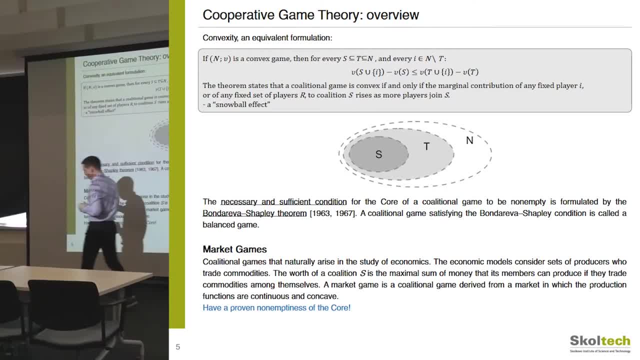 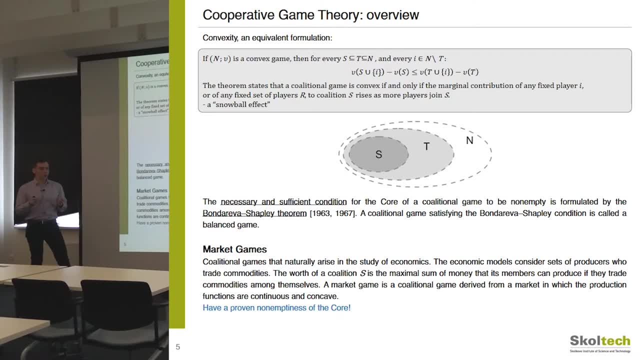 special class of games that is called market games, and market games definition comes from economics, economic studies, when people modeled they considered set of producers, and producers collaborate to trade some commodity and usually when you trade more commodity you get more benefits, so it becomes optimal to trade a. 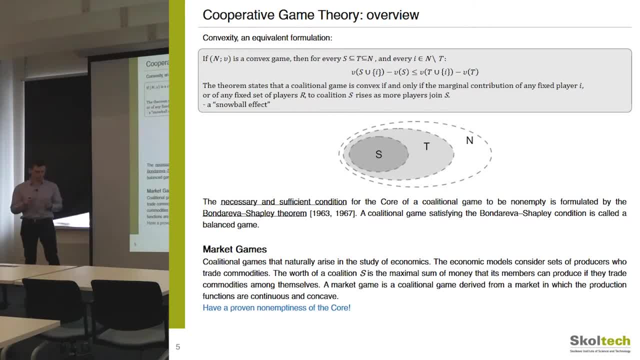 as much as you can. and it is proven that if, if producers have certain cost functions- if I'm not mistaking, convex, con cost functions- it is proven that such games, market games, always have a non empty core. so you also may check: is your game a market game or not? and also let me recall some solution concepts. 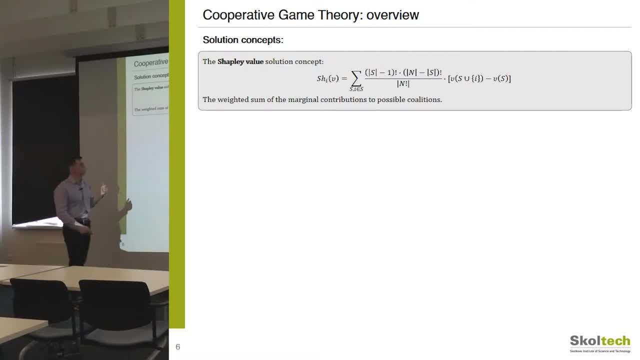 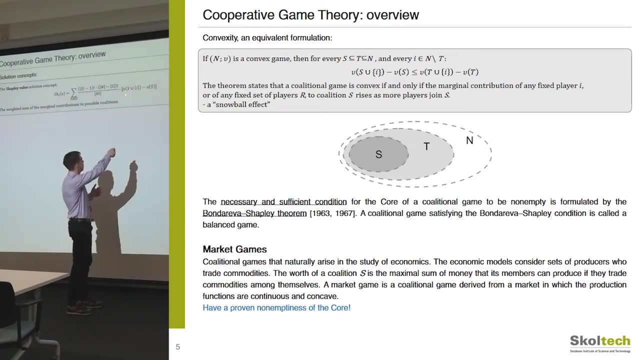 that we discussed the Shapley value, the most popular solution concept that considers marginal contribution of each player to each possible coalition. you may see here the difference called the value of collision with player I minus the value without player I, and we calculate by this formula the weighted. 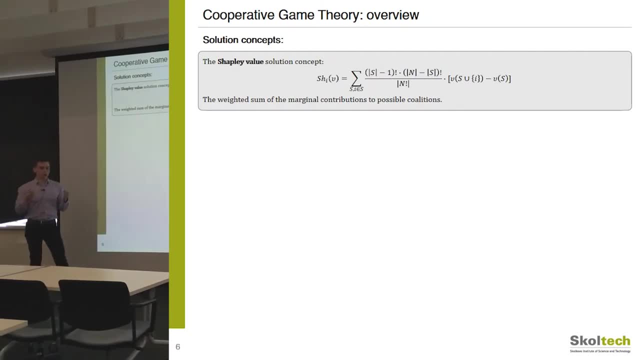 sum of the contributions and therefore we may just plug in the information that we have about a game and get the allocation solution by the shape of value and also I mentioned the new clear loose. it is not such a straightforward approach. it is based on the excess of a coalition, the difference. 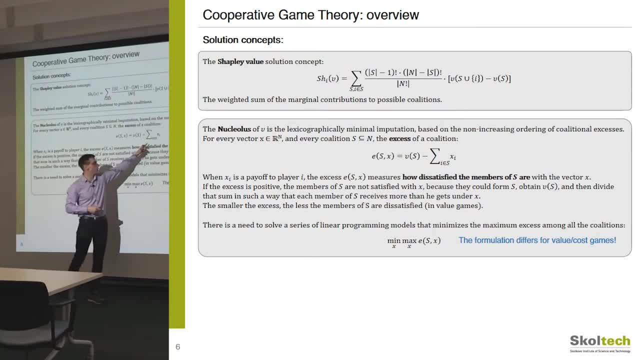 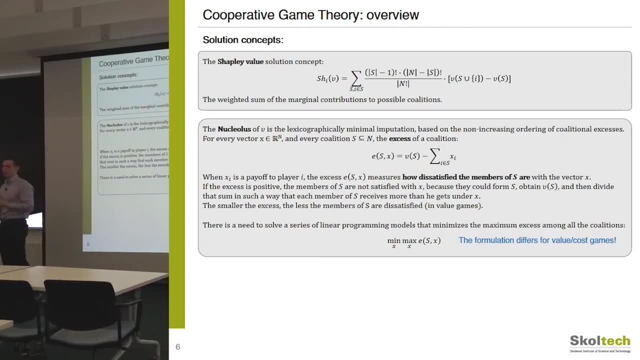 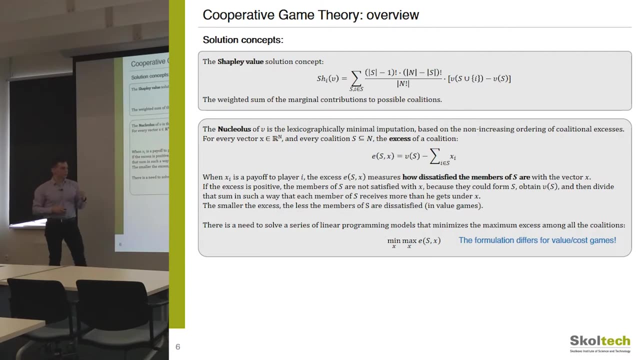 between what collision has on its own minus what it is allocated to the players of this coalition. And in order to calculate Nucleolus, you need to combine a set, a series of linear optimization programs where you want to minimize the dissatisfaction of the most dissatisfied coalitions. 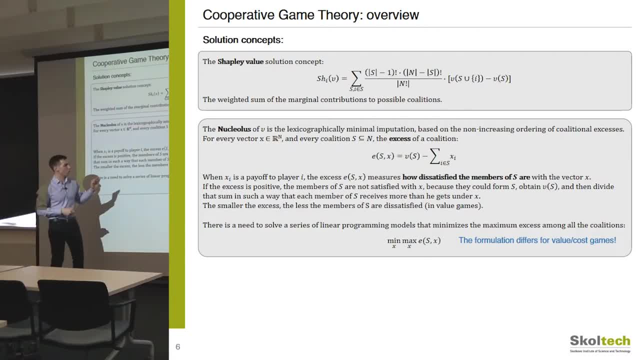 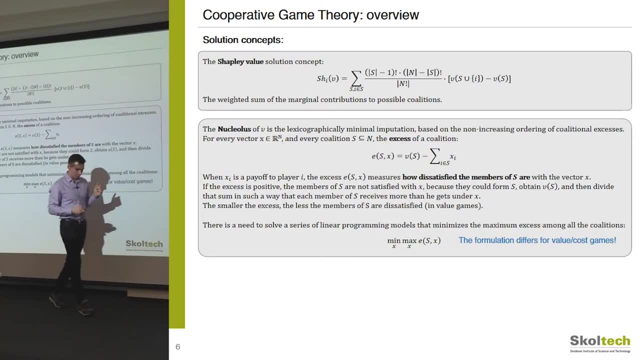 And this approach is also not so straightforward. Moreover, this formulation depends on, again, what do you have, a value game or a cost game? And therefore I recommend you, if you by any chance want to calculate Nucleolus. 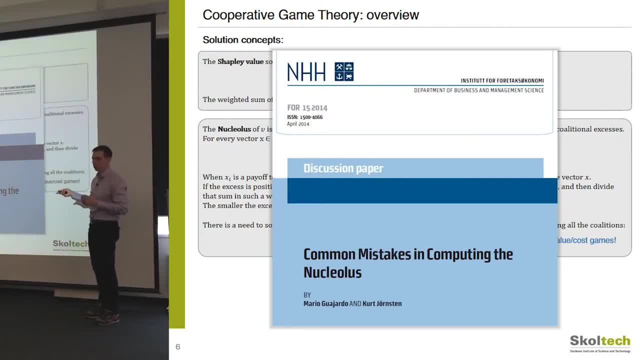 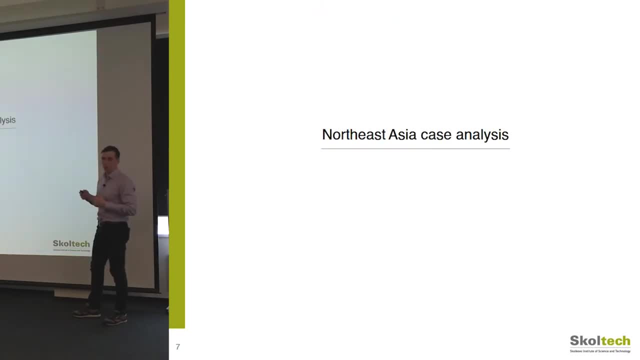 refer to this paper. I think it's rather funny- common mistakes in computing the Nucleolus, but it helped me a lot not to repeat some mistakes. Okay, I think that's all about overview of cooperative game theory solution concepts, And now let's go to the Northeast Asia case study. 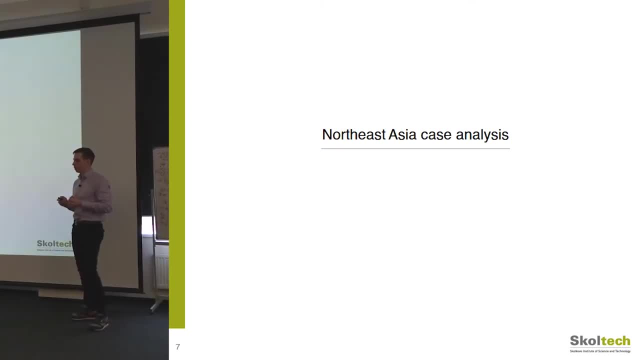 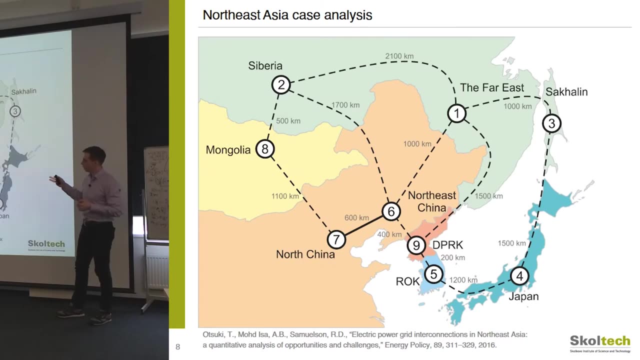 This is the main case that I study in my thesis, and it is also often called the Asian super grid in the media. So this is the scheme that we study. You may see six countries here: Russia, Mongolia, China, North and South Koreas and Japan. 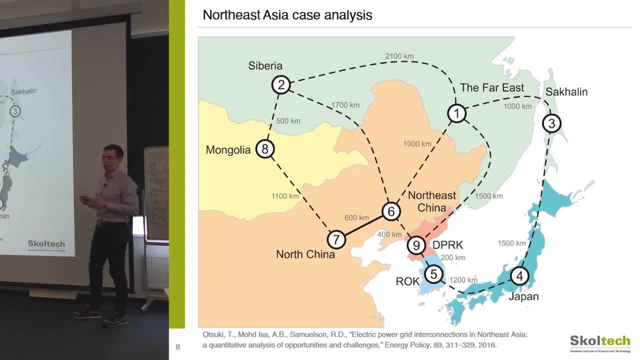 We gathered a lot of information about this case from some papers, technical reports, our own engineering judgment As a reference. the closest study, I think was done in 2016 by Takashi Atsuki. He also wrote a paper in Energy Policy. 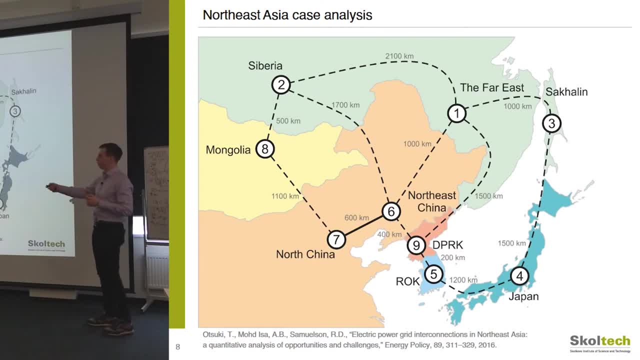 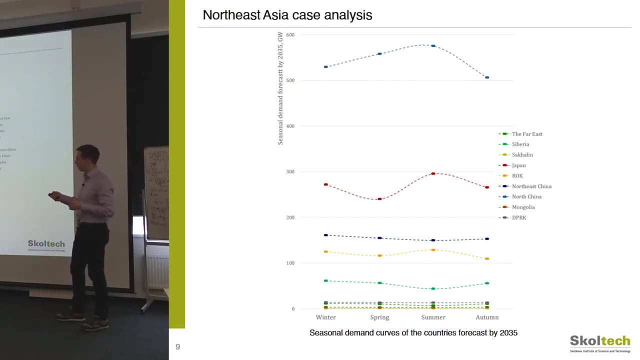 about interconnections in the Northeast Asia And we suggested this dashed line with certain parameters, certain costs that could be optimized among the countries. And first let's briefly talk about the data. This is the forecast that we found for these nine power systems for 2035.. 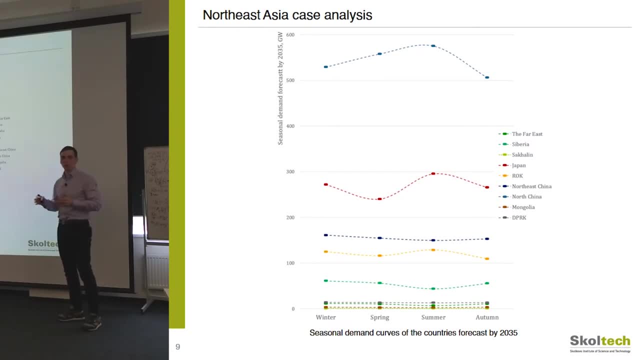 And what you may see here, that consumption in these power systems differs a lot. For example, the highest consumption is in North China, I believe, And you may see that it's almost reached 600 gigawatts. It's a lot compared to other systems. 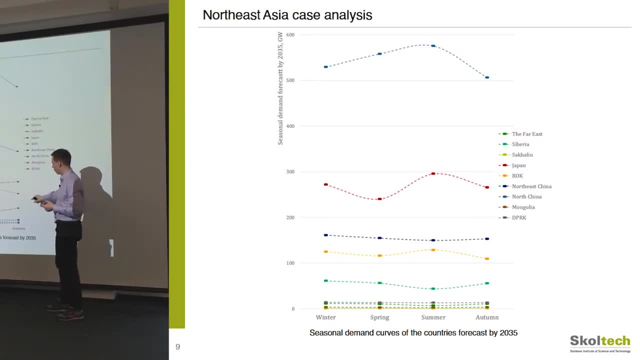 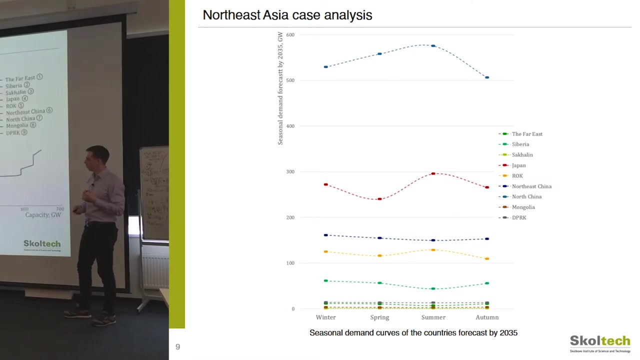 The red line represents Japan and other countries. you may see see that three power systems of Russia that are considered here: the Far East, Siberia and Sakhalin. they are not so significant in terms of capacity. then we identified generation sources in each of the power systems and composed this: 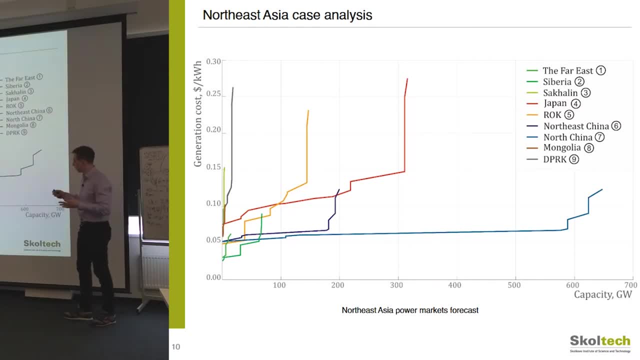 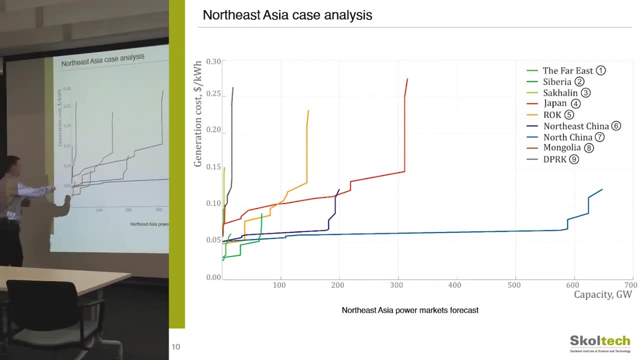 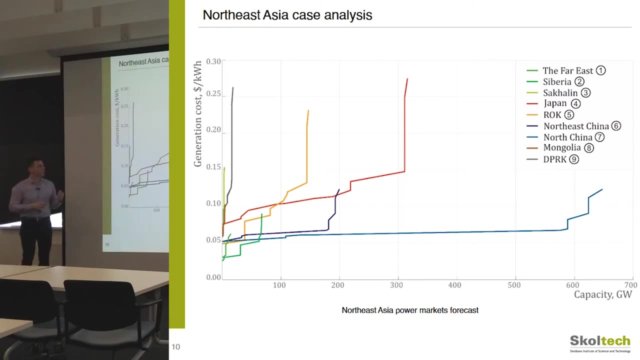 approximation of the cost functions. and here again you may see how big is the cost function, the capacity of North China and this red curve representing Japan. you may see that it is higher than anyone else. this means that in our, that we suppose, in our conditions, that Japan will have the highest electricity price. 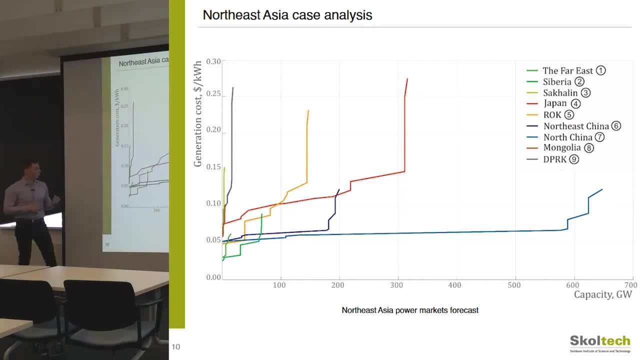 in the region and it will be the main power importer. and this small green power systems is Russia not so significant, but you may notice that it is supposed that because of the Siberian hydro power plants, Russia will have the lowest electricity cost and therefore it will be the main power exporter. okay, 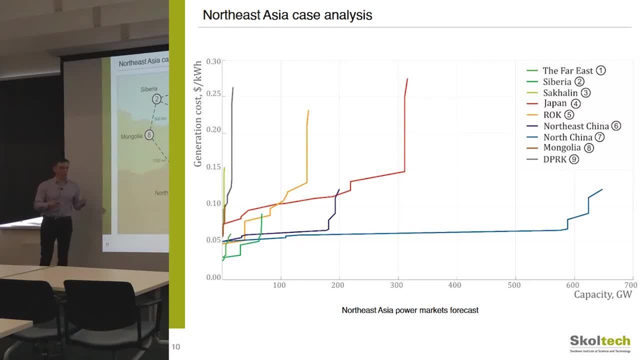 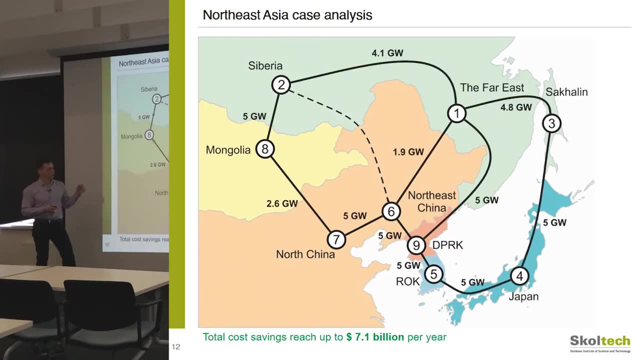 then we plug in this information to the optimization model and we want to solve the transmission expansion planning and this is the result for the grant coalition. that means that all the six countries cooperate and they agree on building the optimal power lines. so you may see the capacity of the lines that are built and 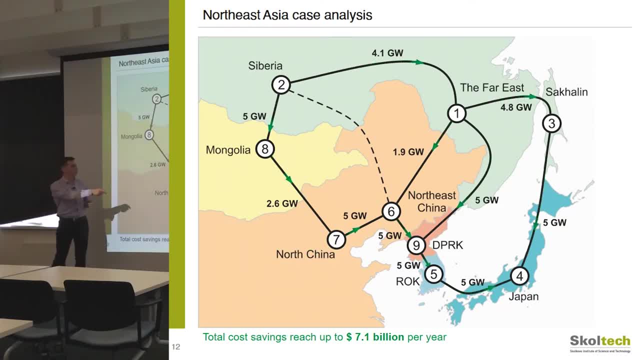 powerful directions. some of the power flows are reversible. for example, in the line 1- 6, you may see that depending on the season the power may may flow in both directions. but some power lines are built up to the maximum and it is seen that there is a 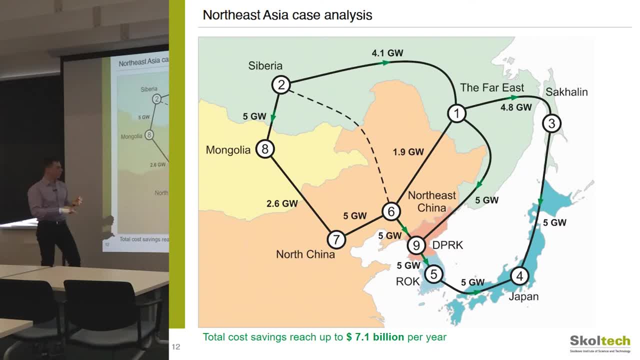 strict power flow towards the Korean peninsula and Japan and when we compare the capacities of those lines, they're not the result of solving some optimization. optimization, yeah, I said. I said the limit: five gigawatts maximum, and you see several lines reach this limits. I think this is. this is a reasonable limit at five GHz, if I'm. 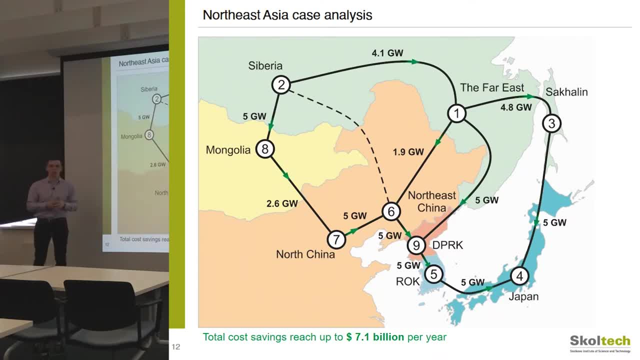 really sure, considering nowadays technologies? yes, and then we just compared the case of no optimization and the grant coalition and the difference in objective functions in cost savings means seven billion dollars per year. but this is for six countries and the question of that we pose here, why we use cooperating in theory, we ask. 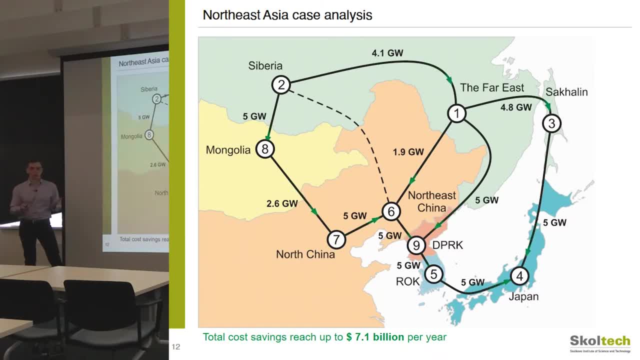 how? how should these savings and these costs be split among the countries? and therefore we introduce players and, as you guess, here are six players, one player per country, like for Russia, Mongolia, China, North and South Korea and Japan, and these players should agree somehow. and the first step, as I explained, 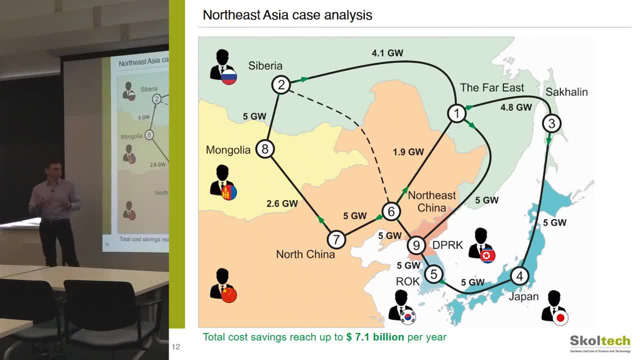 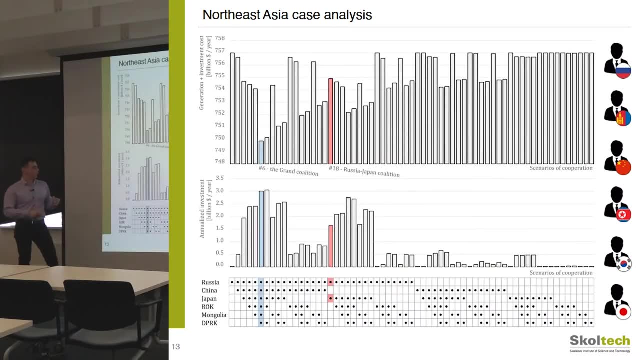 you, we need to describe all possible scenarios, all possible collisions of players, and we can plot this by this bar chart. you may notice that there are 63 possible scenarios, as we discussed two to the power of six minus one, and this plot itself shows us a lot of information. 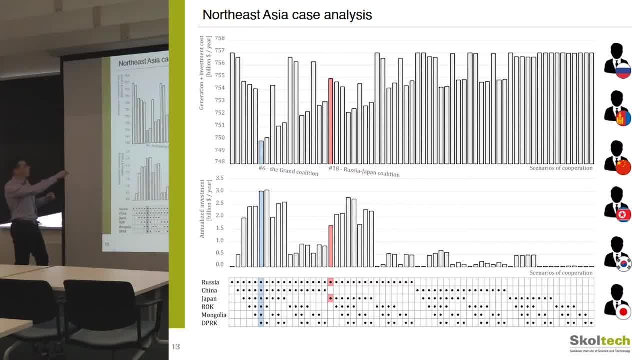 the upper chart shows us generation plus investment cost per year. so basically this is our objective function for each possible scenario. here we see only investment without generation cost, and below we see all possible combinations of players in the 63 coalitions and we may study a scenario. 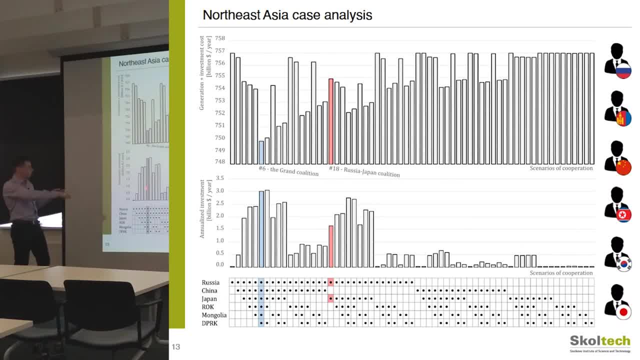 by scenario in order to get some insights. for example, scenario number six: when all players cooperate, the grand coalition is indeed the best, the least cost scenario for the region, but is it a stable cooperation? will the players agree to be in the grand coalition? in order to answer this, we need to consider more scenarios, for example, a bright example here would 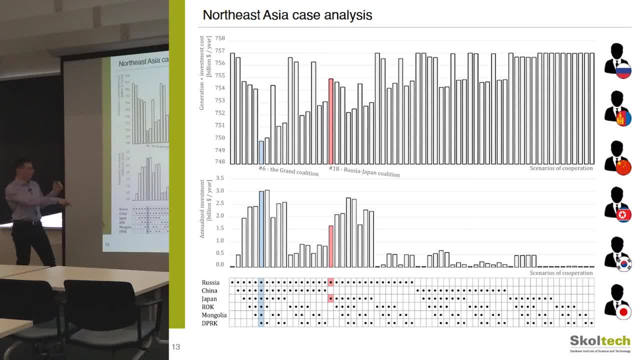 be scenario number 18: Russia and Japan only. you may see only Russia and Japan cooperate here and they get less savings. but they need to split their savings only among two of them, and maybe it will be more beneficial for them to not cooperate in the grand coalition but only to build. 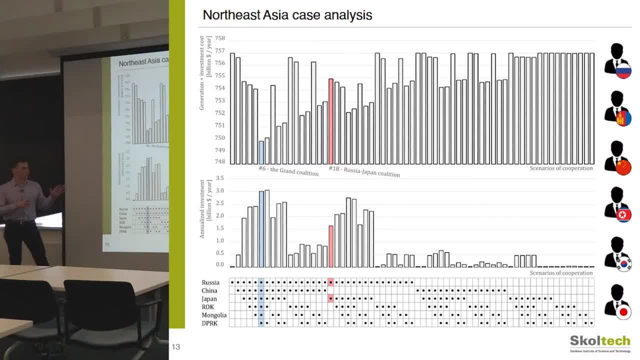 um, this bilateral interconnection, and this is the issues that we will be considering, uh, next, and also, you may consider all the scenarios, like by countries, for example: uh, what coalitions do Russia? few more slides, please. okay, I want to say that there are many ways to analyze this figure, and 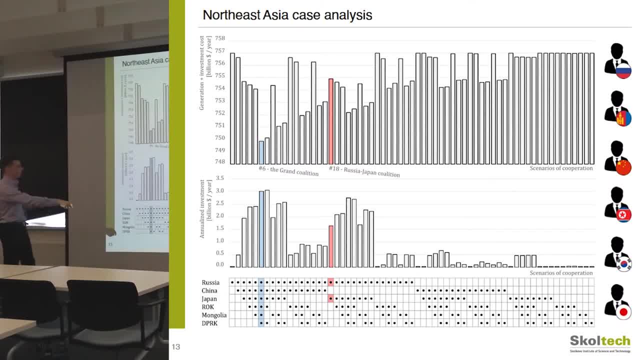 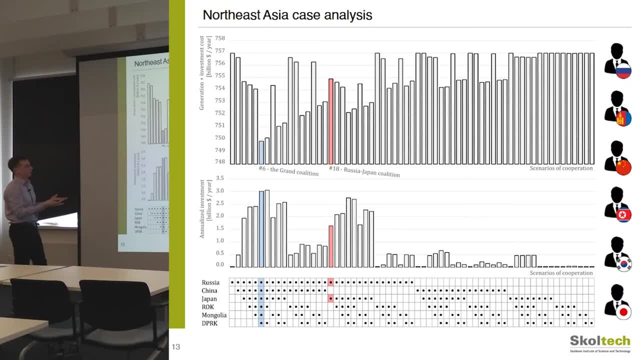 get some insights. for example, we can consider all coalitions that Russia participate and see uh. and if Russia uh breaks this agreement, these coalitions uh simply do not exist there. they become infeasible. and you may see that Russia is an influential player, right, but then you can exclude. 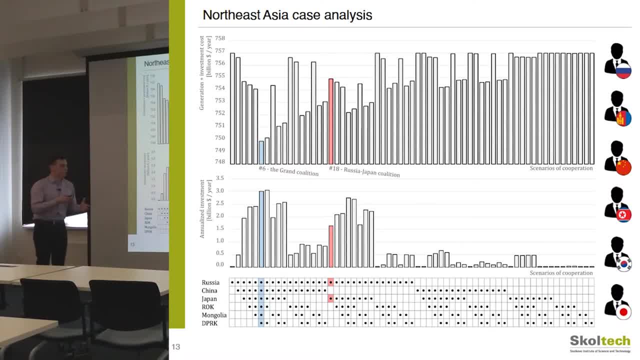 coalitions with Mongolia and see that not so much will change. and by doing this analytically you may conclude what countries have what influence on the cooperation. but there is no need to do this manually. you can plug in this information into Shepley value, for example, and get the following: 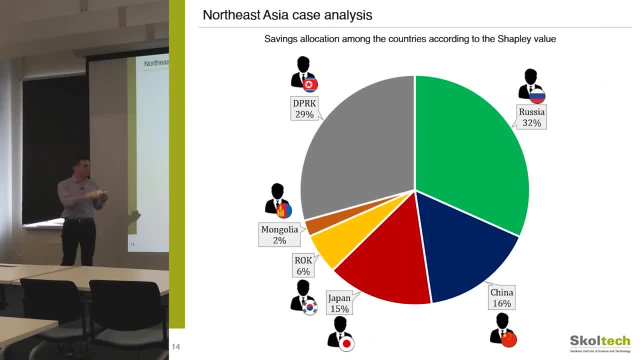 allocation of savings. and here you see that, indeed, Russia gets 32 percent of savings, and we can say that Russia is a very influential player in this coalition. but an interesting thing is that the next most influential player is North Korea, with 29 percent of all savings. and how is it possible? this is a small. 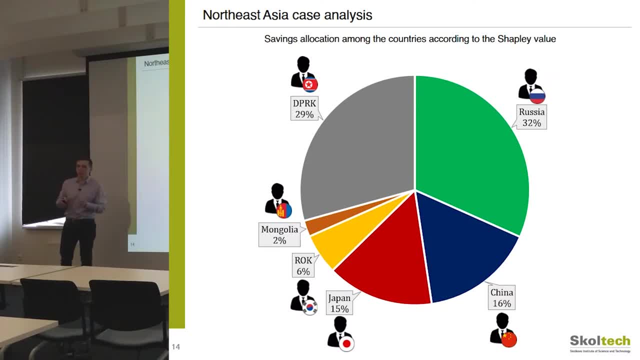 system with not the cheapest electricity. and do you have any ideas why North Korea is such an influential player here? maybe for Korea? yes, right. so Cooperative game Theory, that doesn't lie to us. it shows us the true conditions and we see here that North Korea has not economic advantage, but it has topological Advantage. 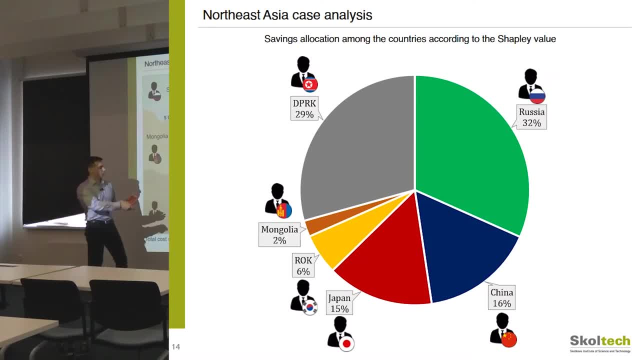 if it breaks an agreement, there will be no power flows to Korean Peninsula and Japan and therefore, even though this is a comparative, the small power system, it turns out that North Korea is very influential and very important player. that should be played accordingly. Yeah, but there are other constraints that you impose, like 5 gigawatts. yeah, 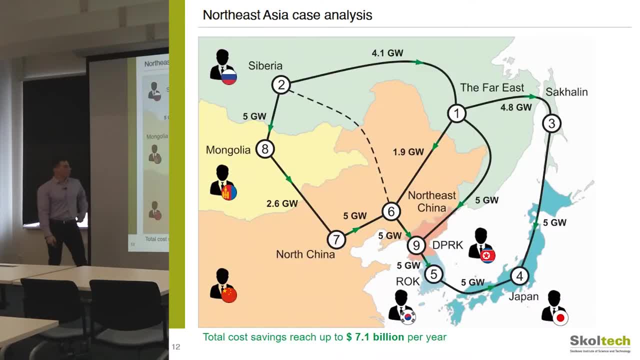 So if you return to the map, so you see, if North Korea breaks the agreement, then the line 1-9 doesn't exist. What you can do instead is you can build another parallel line to Japan and if you consider that possibility, then maybe North Korea. 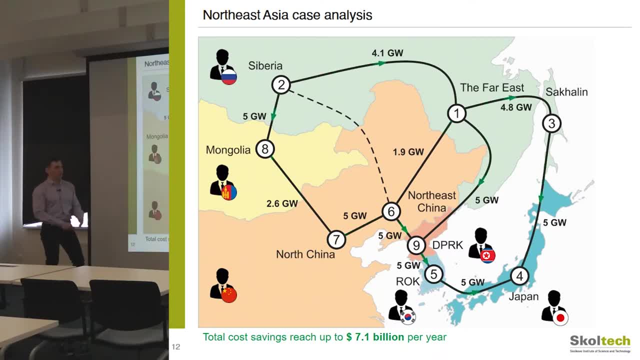 becomes not so influential. Yes, This is another way of analyzing this. You may just imagine what happens if China says, okay, but there is also a possibility of building a line here, And if you change this, the cooperation will change. But yeah, we analyze. 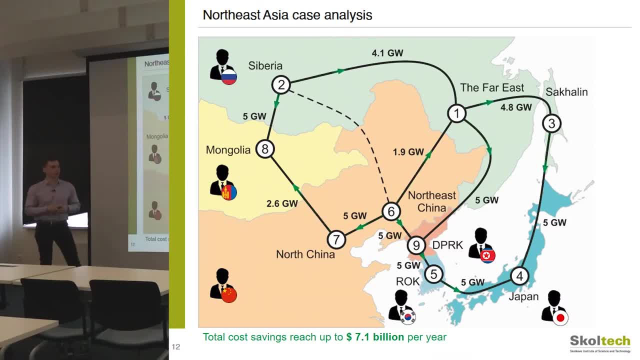 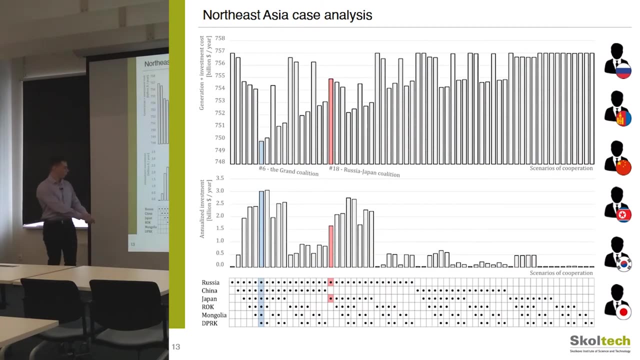 these given conditions, but there are many ways of changing the data. Okay, So let me ask about these bridges. Yes, What is the scenario when you have only one load per hole, One dot? Okay, the first one, only Russia. 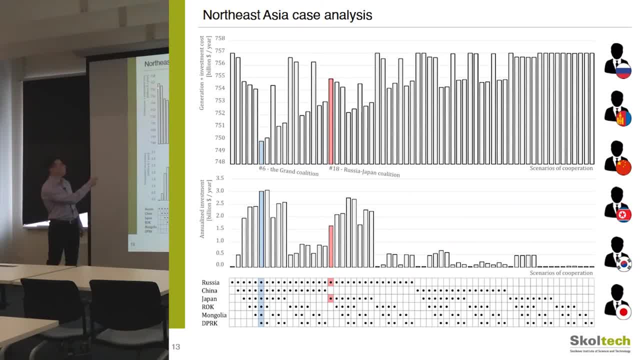 Yeah, the first one, Yeah, what does it mean? This means no cooperation, I think, no investment and no savings, All these scenarios. so you have the last one. Yes, The last one means only No, no, no, no. The last ones are, for example, 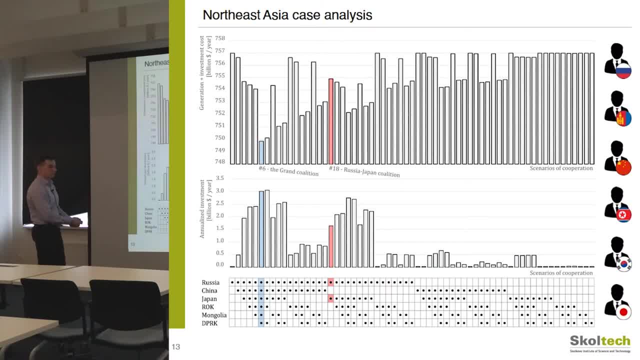 cooperation between Mongolia and North Korea. just an empty set. Oh, the very last one, The very one, no only one, means no cooperation. Yeah, But So it is equal to the first one. Some of your scenarios don't have cooperation if there are two countries that are separated. 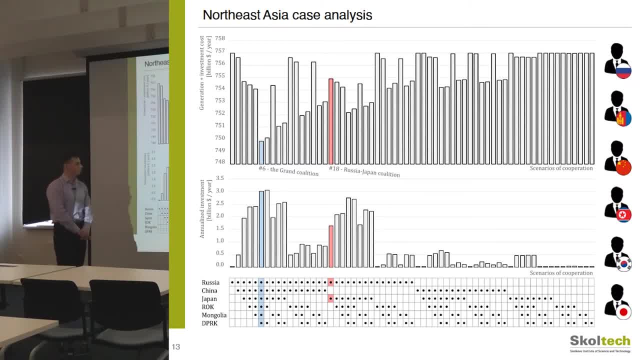 geographically Also, Like the last draw. you see, for example, Mongolia and DPRK, It doesn't matter if they cooperate, Right, It's just an empty set. The model sees this topology, that they, we say they cooperate, but the model says: 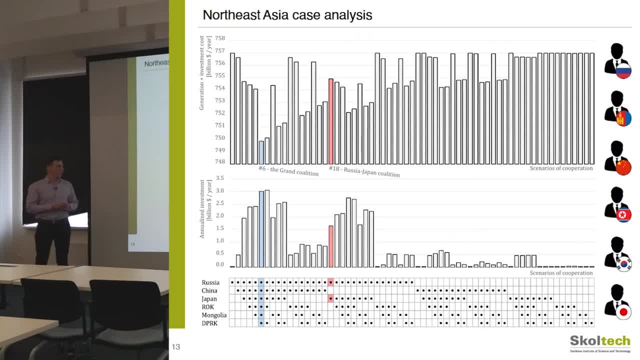 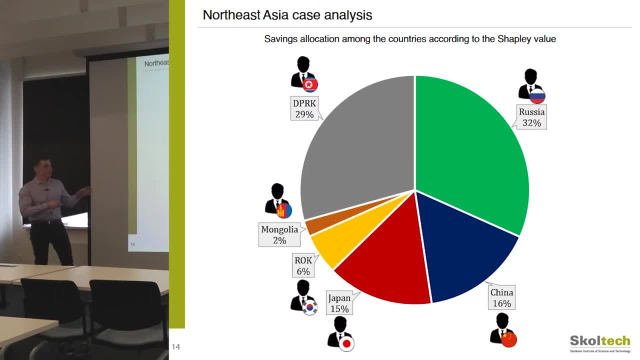 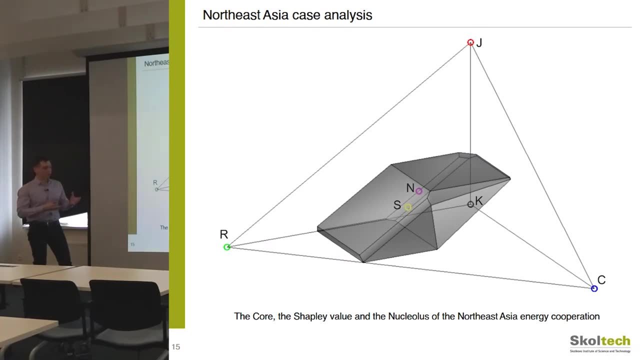 But it's nothing. Savings zero means Yeah, Nothing happens. No cooperation: Okay. So the application that showed us bargaining power. we see Russia is a good power exporter gets some savings. North Korea is also important, And then we can plot this to analyze the core of the game. 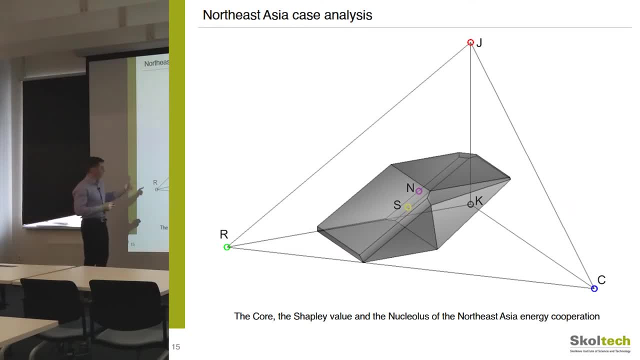 And you remember the barocentric coordinates, meaning that certain vertex for a player- for example, this is Russia- means that Russia here gets all the savings, And the further we move in this space from the point R, the player gets less savings. 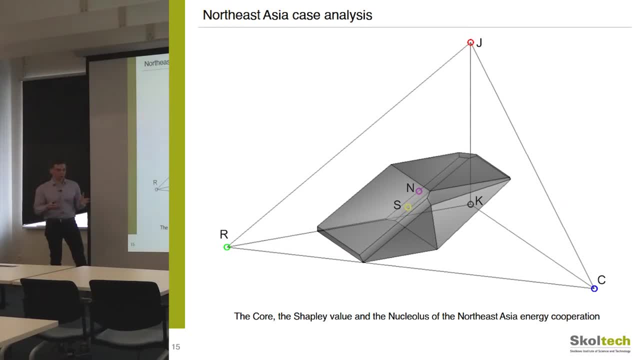 And we cannot plot six players' game in the 3D scene. But what we can do, we can fix less influential players in the Shepley value point, for example, and plot the remaining ones. So here you see: Russia, North Korea, China and Japan. 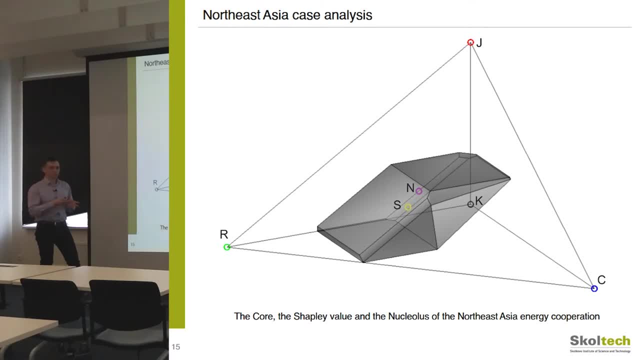 And you may see that the core is large enough. There is enough space for bargaining, And the allocation solutions, the Shepley value and the Nucleolus lie inside the core and they are not close enough to the borders. So we may say that this certain cooperation is stable. 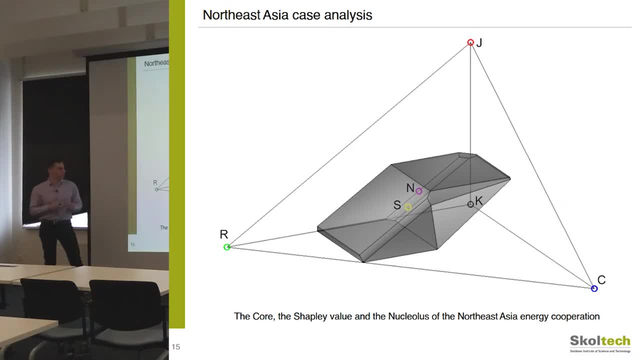 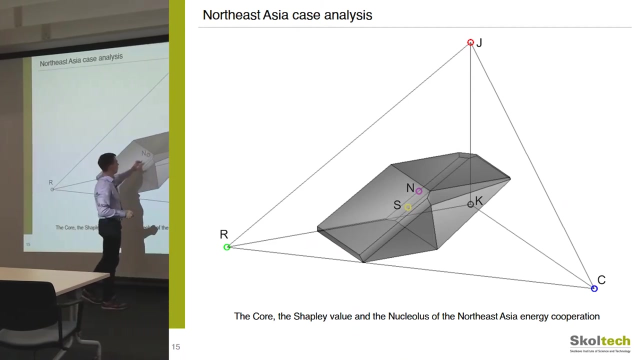 Even under certain data perturbations. And there are many ways also to analyze this figure by analyzing certain projections. Imagine that you are looking at this figure from the point C, So you are working in this dimension- Korea, Japan, Russia. What you will see? you will see this parallelogram, I would say, hanging over the point of North Korea. 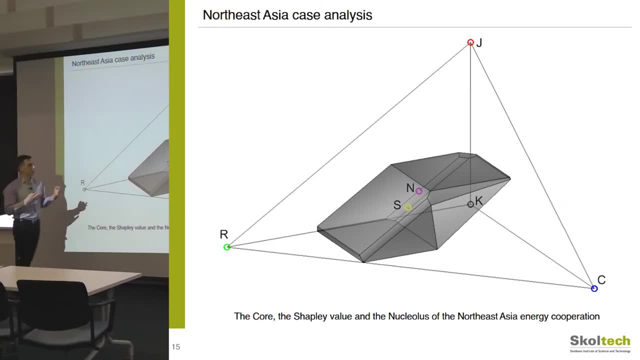 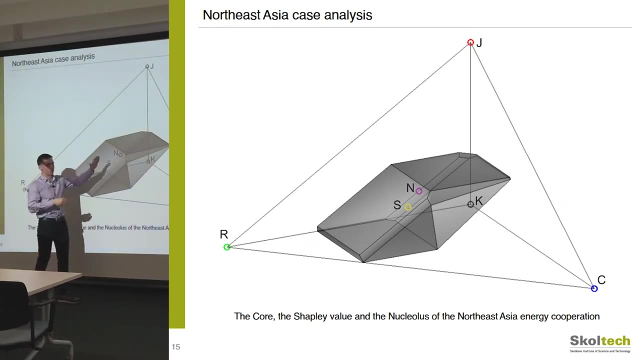 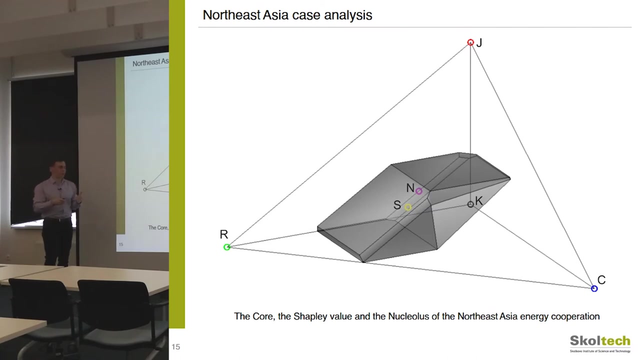 And how you can interpret this. you may say that North Korea is not getting more power in this cooperation because Russia exists, Because coalition Russia-Japan exists, This condition exists, This restriction, And therefore Korea cannot be the most influential player, because there is also an option of exporting power from Russia to Japan. 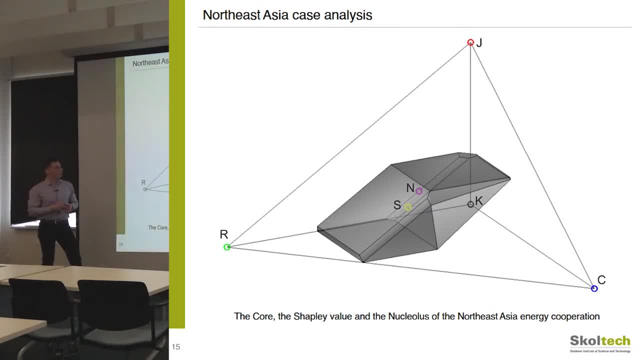 So you may get really interesting insights from the figures of the core And some people asked me about plotting such figures And I would say I would recommend you to use the package TUG lab for MATLAB, I think from 2004.. And this package means transferable utility games lab. 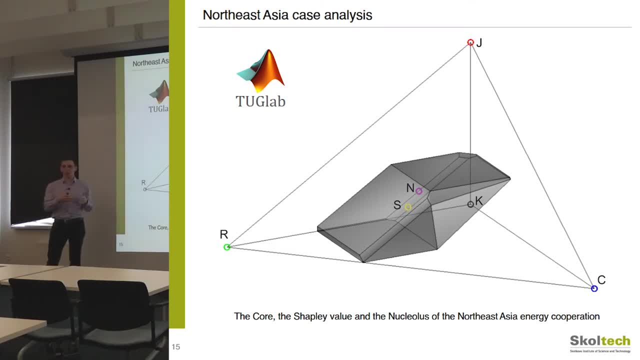 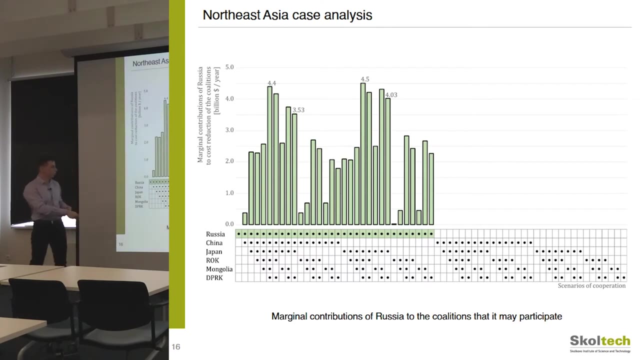 And if you give to this package your function for three or four players- cooperative game- it would automatically plot the figures for you, some allocation solutions. So I recommend you to use this package. Okay, And another interesting plot: The original contributions of Russia to the coalitions that it may participate. 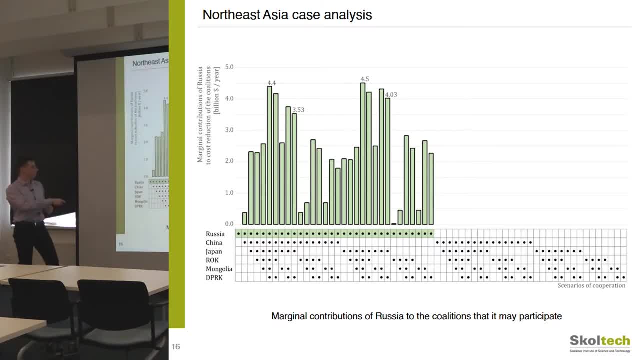 So you remember the list of possible combinations, And here we highlight the coalitions with Russia. So here nothing exists, because Russia doesn't participate in these coalitions. And let's study this particular plot. We can compare certain coalitions, For example the Grand Coalition and the same coalition, but without China. And we see that Russia contributes $4.4 billion to this coalition, But $4.5 billion to this coalition. And another situation could be the coalition of Russia, China, Japan and North Korea And the same coalition but without China. 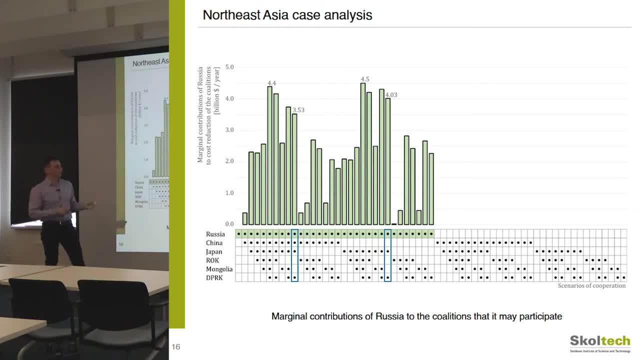 And again, Russia contributes more to the coalition with less players, And the question is why this happens and what does this mean to us? And, as you guessed previously, this means that the game is not convex, And this is the bad news for our analysis. 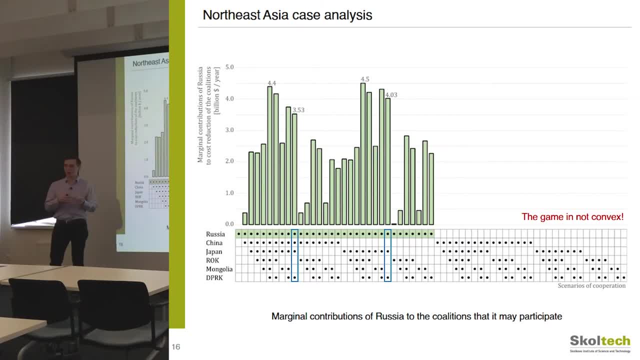 Even though we study power markets optimization, the game turns out not to be convex, Probably because of the cost functions and the nature of transmission, expansion, planning, the limits on the power flows. So we should be careful when studying such games because under certain data it is possible that there will be no cooperation. 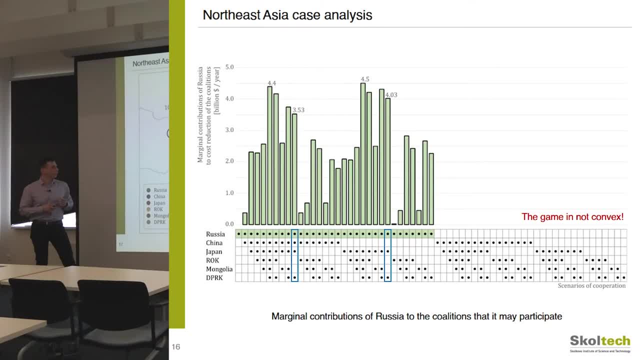 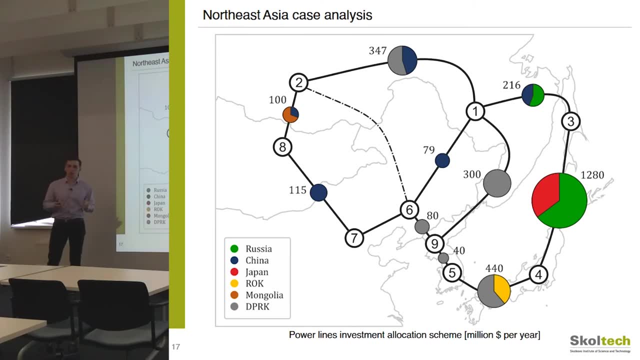 And cooperation would be not stable. Okay, And we need to answer a few more questions for this case study. The first one is: we found some allocation of the savings and of the cost, But can we suggest a solution to the allocation of the cost of each particular of these lines? 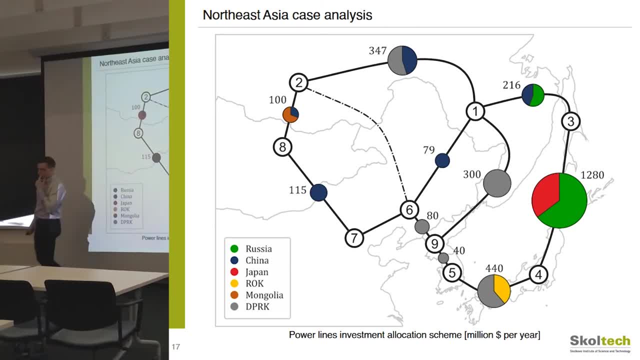 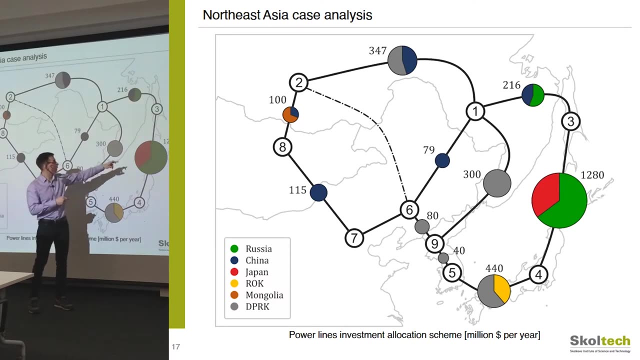 And the problem is that there is no unique solution. There are many combinations of this investment And let's see that, for example, this green volume here means the share that Russia should invest, And we can just say, okay, Russia invests in this line with Japan and a bit in this line with Sakhalin. 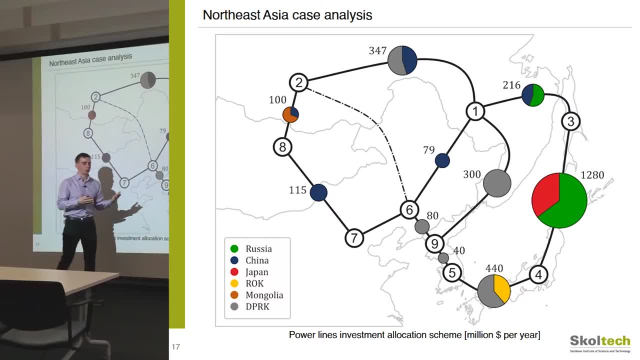 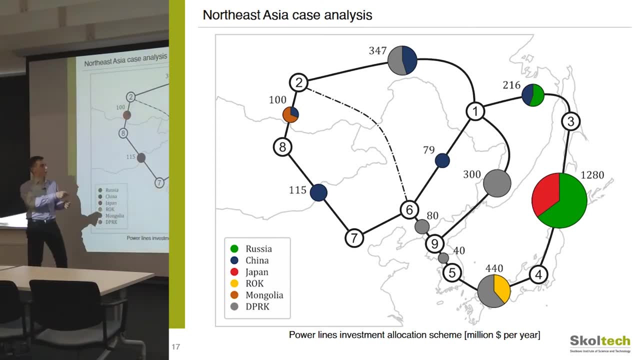 But then Russia has no more money to invest in this, under these consumptions, under the Shapley value solution. And who should invest, therefore, in other lines that are entirely in Russia? And probably the game theory would say that China and North Korea should invest there. 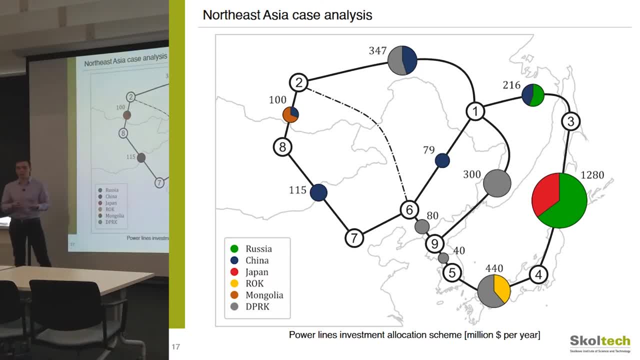 And this result could be fair theoretically, But politically it's almost impossible. And we found this feature And there is a need to developing new mechanisms of cooperation to deal with such issues. What should happen if countries do not want to invest abroad? 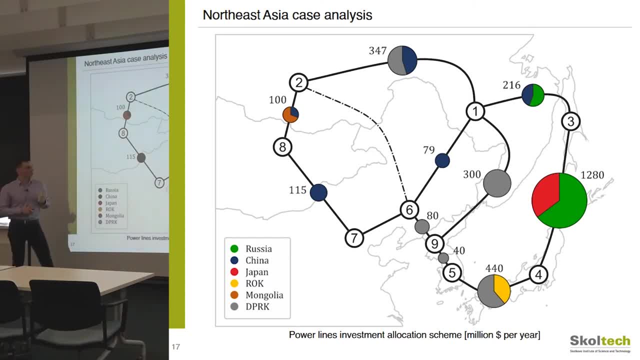 And also, you may wonder why not to implement game theory again and combine multiple games, each cooperative game for each of these lines, Saying that in what scenarios the line participates, what countries are interested in this line, And therefore, again, maybe by Shapley, split the cost of each line. 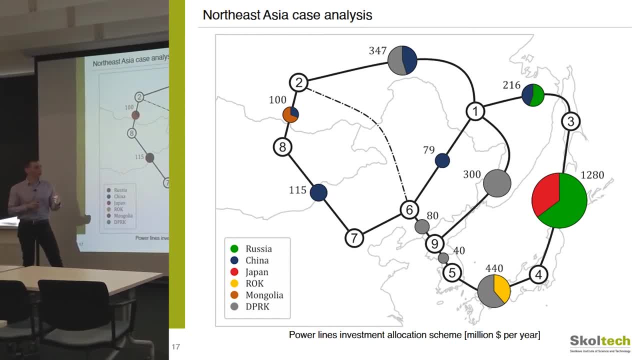 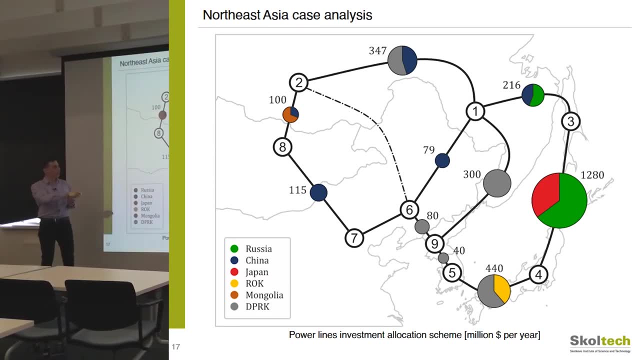 But this wouldn't work because the game is highly non-convex And, as an example, you may see that the line 2-6 is not built at all in this optimization plan Right, But in some sub-coalitions, for example, where there is no line with Mongolia, this line is built to certain capacity. And this could lead to strange results that are not implementable- That some countries should compensate other countries Because they didn't build certain lines, And it's also very disputable. So there is a need to investigate some mechanisms of how to split the cost of each particular line, if you want to answer this question. 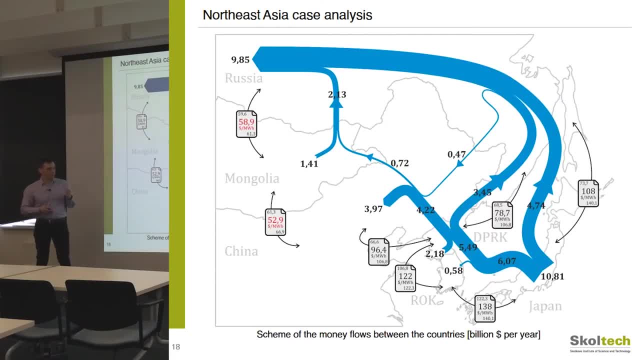 And also, as I said, we calculated the allocation of costs and savings by Shapley value. But remember that the generation cost in Russia increased because Russia starts producing more power And the cost in Japan decreases, So there are some savings happening right in Japan. 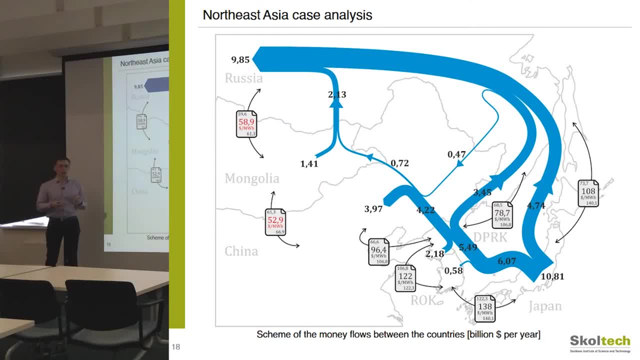 And countries should compensate each other. And the question is: can we calculate the money flows, the ways of compensating the countries? And we even composed another optimization model over the initial one, when we formulated money flows among the countries and marginal costs, And we tried formulating, you see here, bilateral contracts. 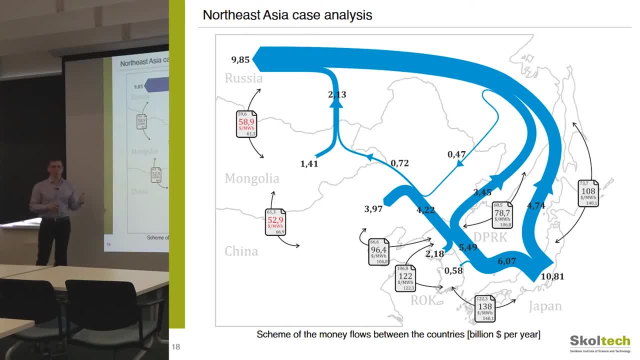 And we found that for this particular case the cost of the money flows was much lower. But for this particular case bilateral contracts would not work, Because game theory and optimization of money flows tells us that there should be some flows of money among the countries. 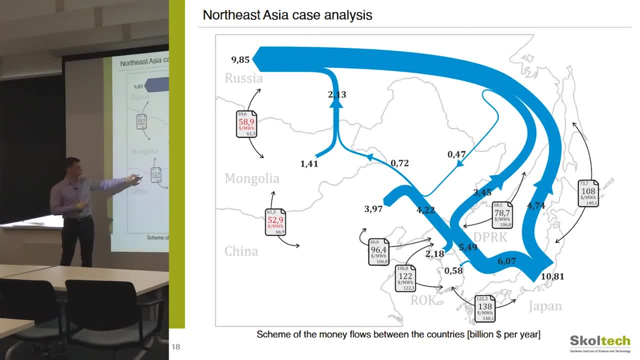 But if we calculate the contracts we will see some strange results. For example, Mongolia is exporting power to China. Its cost is $61.. Marginal cost of China is $66. But game theory says that Mongolia should sell power at the price $52.. 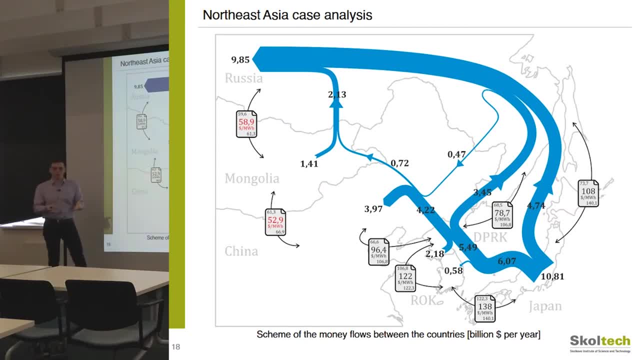 Less than its own cost, And also very disputable results here that show that bilateral contracts would not work if we want to split the savings and compensations by the game theory principles, And the solution could be: if there is a certain coordinator, some intergovernmental entity that would collect all the money and then redistribute it. 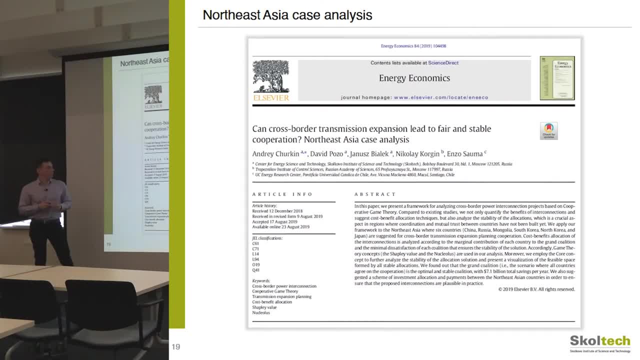 And, yes, we published this paper. It's very interesting. We published this paper in the Energy Economics Journal last year, So I encourage you to read the paper if you are interested in all of these concepts and features that we found here. Okay, 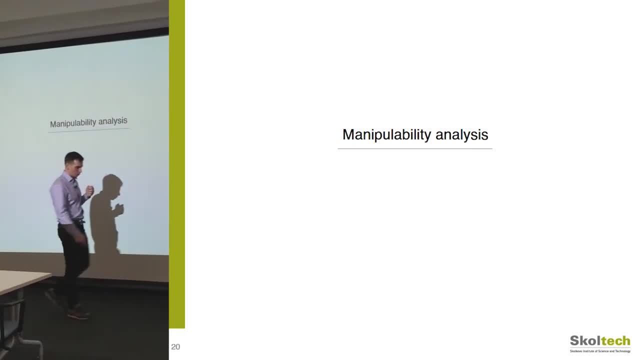 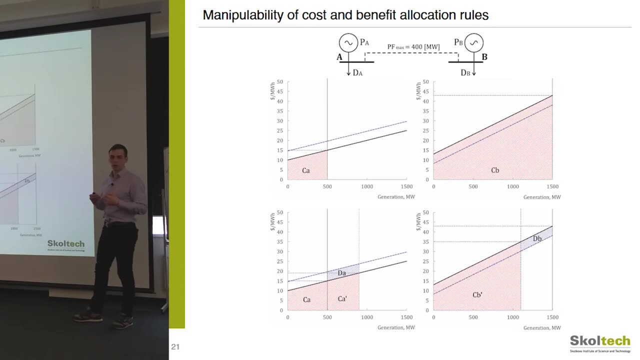 That's all about the Asian Super Green Study, And then next topic that we considered is called manipulability. As you remember, we discussed that game theory highly relies on the accuracy of the information. We know everything about the power systems, their cost, functions and so on. 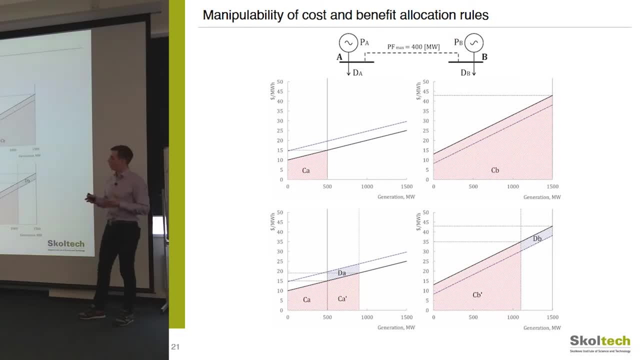 But in reality, we may not know this information And, moreover, some players may try, we can say behave strategically or cheat. They can submit different cost functions And recall these two power systems- example from the previous lecture: The system A with cheap electricity cost and system B with more expensive electricity cost. 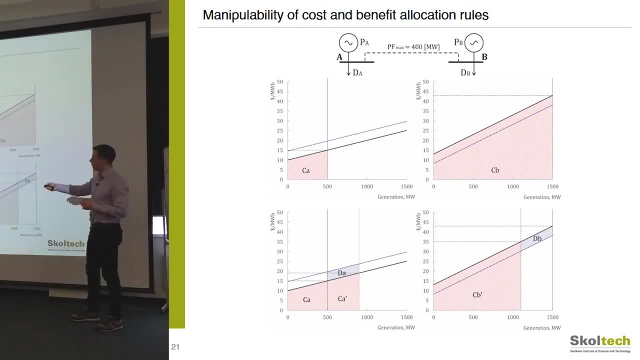 And they are going to build a 400 megawatt line And these bold black lines represent their true cost functions. But system A, for example, may say that: okay, I agree to cooperate with you. We are going to use Shapley value or any technique you want. 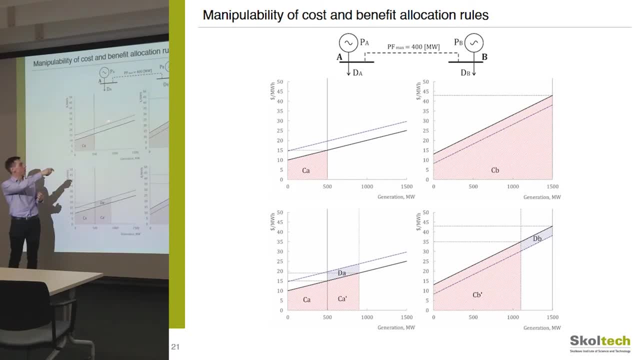 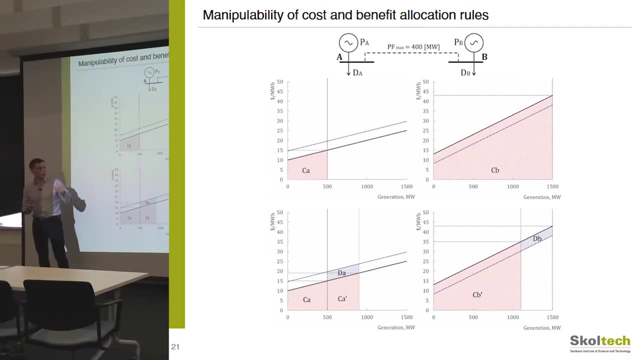 But you know my cost function is not this, It is a bit higher. In other words, system A says that I'm not such a cheap power system. My cost is higher. And what happens? if they cooperate on these conditions, They will get some savings. 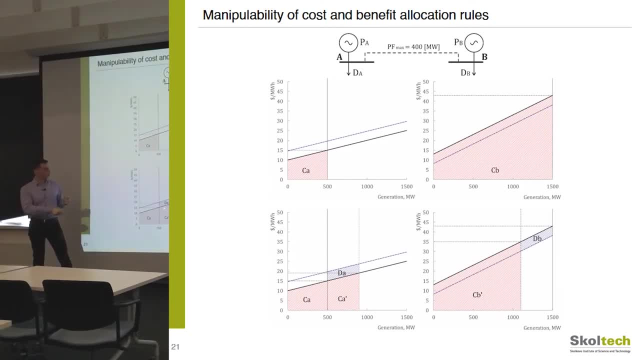 They will allocate them by the Shapley value. But system A will end up with having some additional benefits. We can call it delusion, volume of savings or something, And the same works for power importers. System B may say: I'm not such an expensive power system. 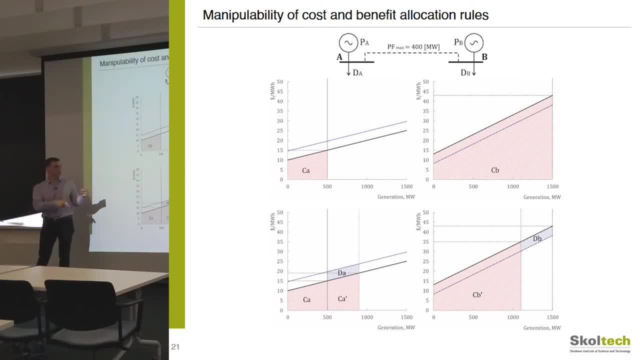 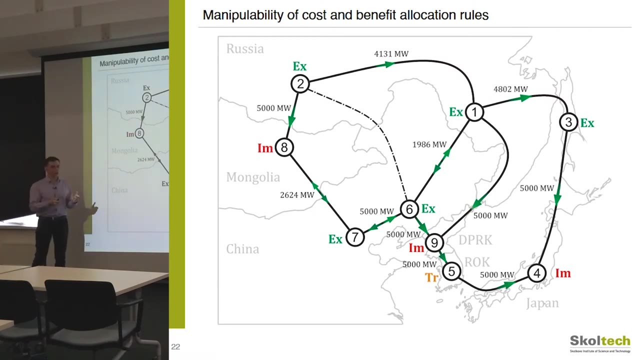 My cost is much less, And let's cooperate using this data And therefore I'm ending up having some hidden benefits. And this is again the scheme of the Asian super grid, And here I highlighted the roles of the players in the cooperation that we got: power importers, exporters. Japan, the main power importer. 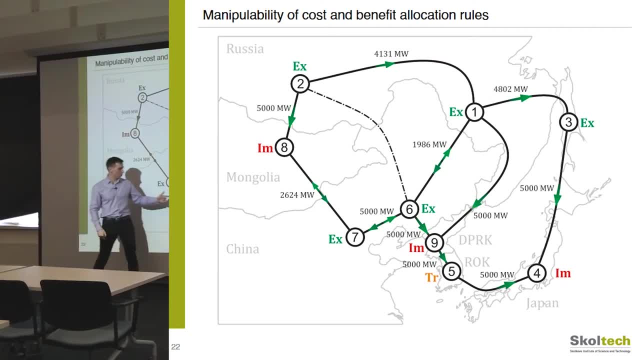 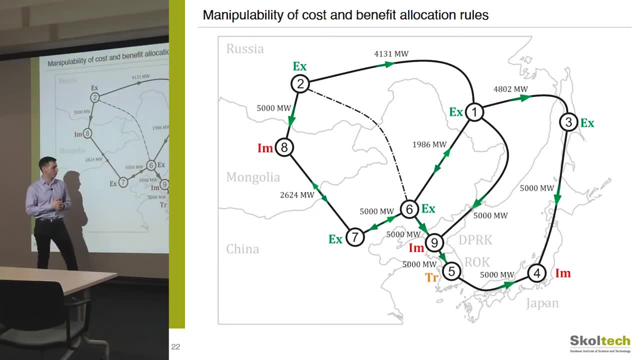 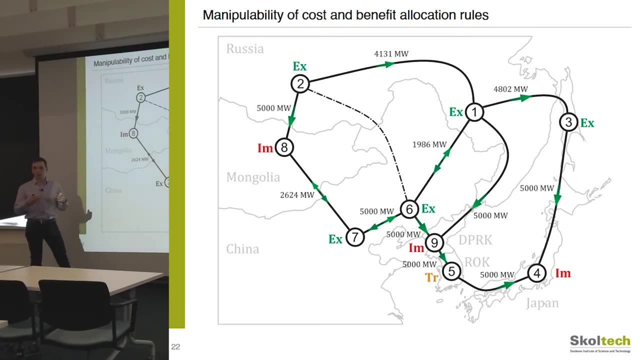 And please notice that North Korea, under this optimization, is a transfer country, So it simply transfers power towards a more expensive Japanese power system And it is paid for this according to game theory. So let's see what happens. If these players start behaving strategically, they start changing their claimed cost functions. 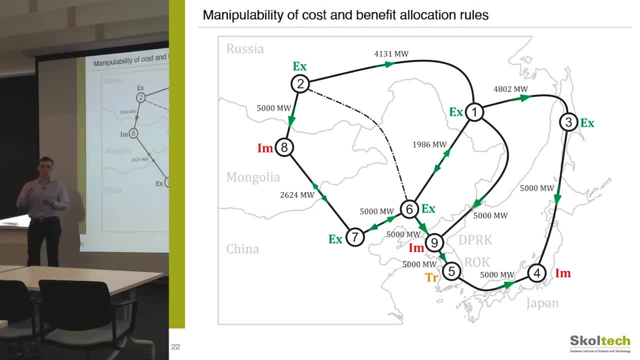 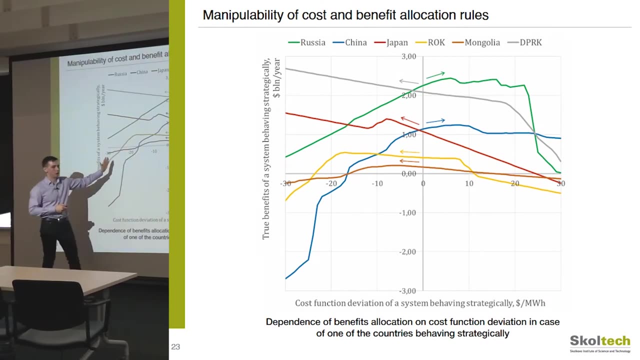 And, as we discussed, Russia should probably increase its cost function bid And Japan should pretend that it is not such an expensive power system. And here we see the plots. On the horizontal axis we see the cost function deviations. If we do it to the left, this means that the country submits the lowered cost function. 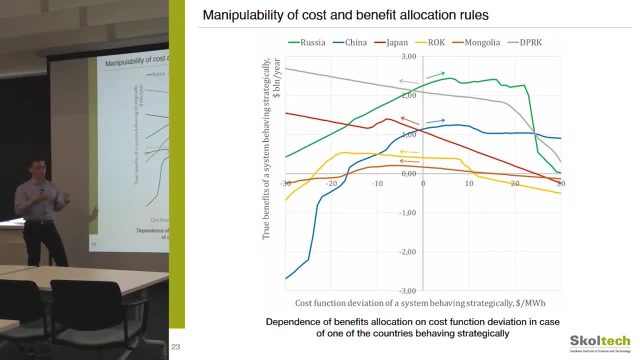 And if we do it to the right, this means that the country pretends to have a higher electricity cost. And vertical axis means savings allocation, the final savings that the countries get. We can take a look at Russia first, the green line- and see that indeed there is this green arrow. 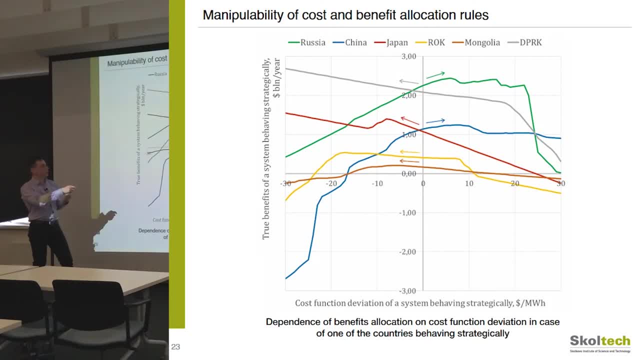 It is beneficial for Russia to claim that its cost is a bit higher. But then something strange happens. You see that this cost is not growing. It starts somehow swinging here, It goes down, And my question to you is: why do you think this happens? 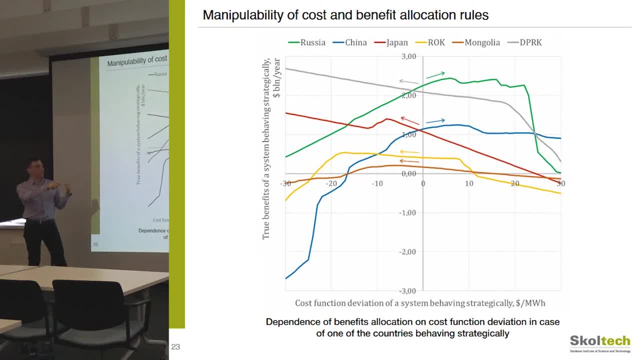 Why this allocation of savings to Russia is not growing like this steadily, Why it starts decreasing. So the export amounts start to decrease because, according to the new distribution, it's not beneficial to buy from Russia. Yes, because Russia is not the only power exporter in this region. 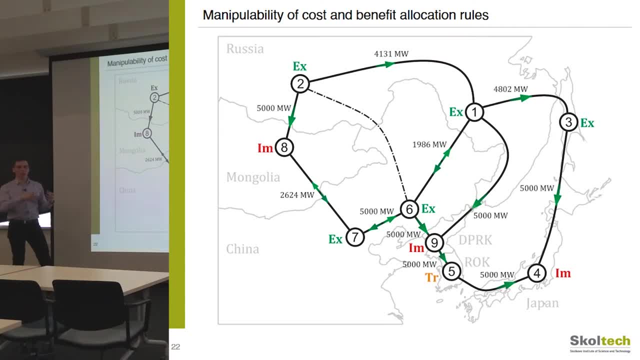 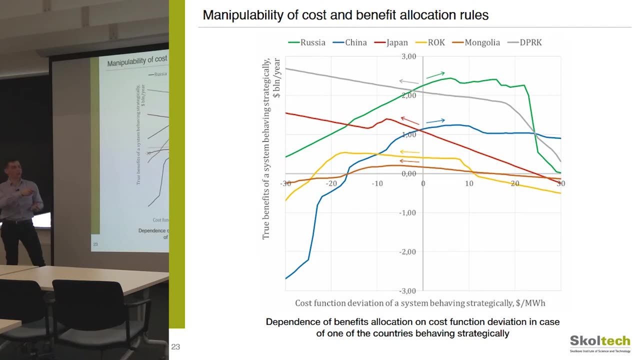 And if Russia starts deviating a lot from its true cost, pretending that it is expensive a lot, then nearby we have Chinese power systems. It runs out of its market power, It is losing the share of market right And it is an interesting result that we see that it's not beneficial to cheat infinitely. 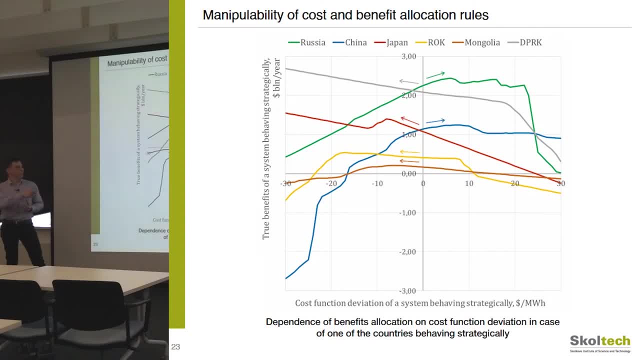 Yeah, cheat a lot And we plot these curves for all the countries. You may also see Japan, the reverse figure. Japan pretends that it is not so expensive. But here we also see an interesting figure. There is an interesting bend here. 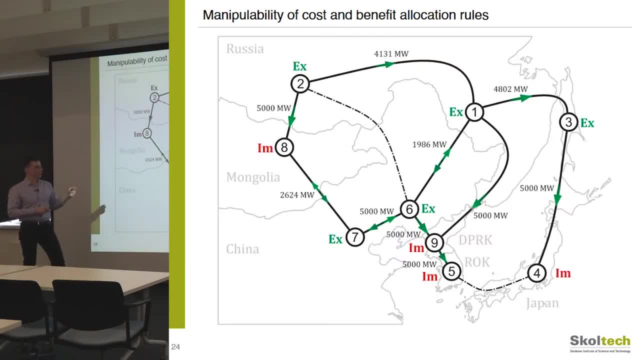 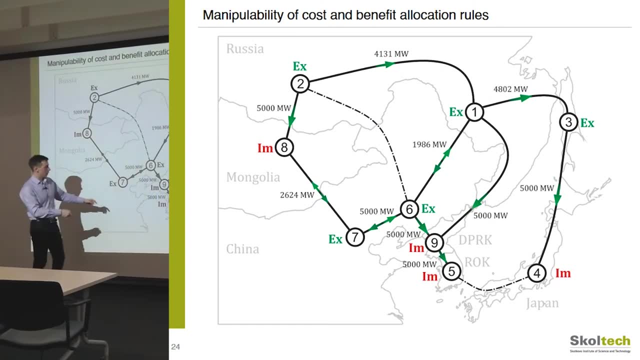 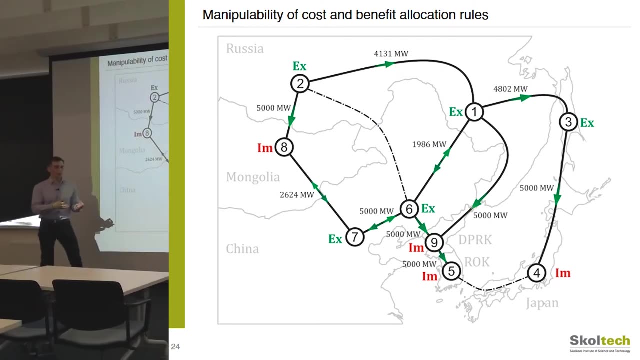 And I can explain why this happens. So this is the figure. when Japanese power system deviates a lot, It pretends that it is not so expensive. And what happens? that this line 5-4 between Korea and Japan, it disappears Because it is not optimal anymore to build undersea cable with the countries that have equal marginal prices. 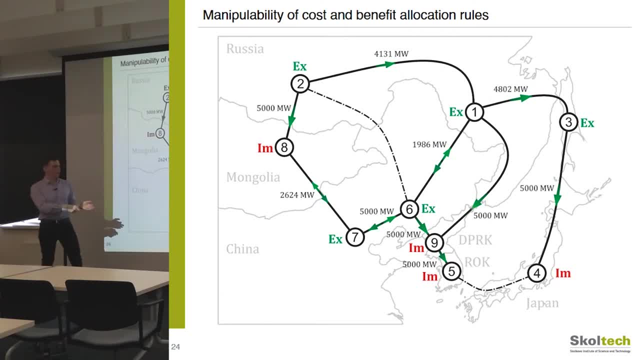 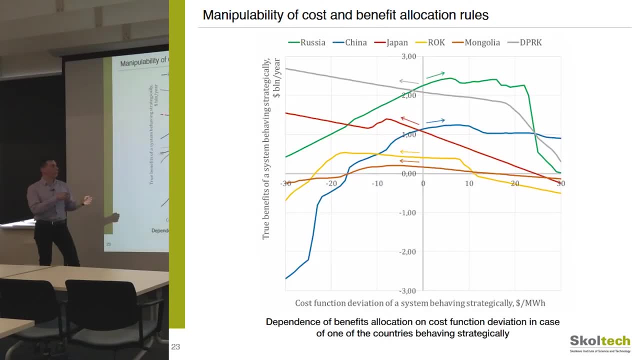 But we can think that if the line, the entire line 5-4, is lost, that the cooperation should be much worse. But for Japan, look, the savings of Japan continue increasing And this is an interesting insight that tells us that for some countries, 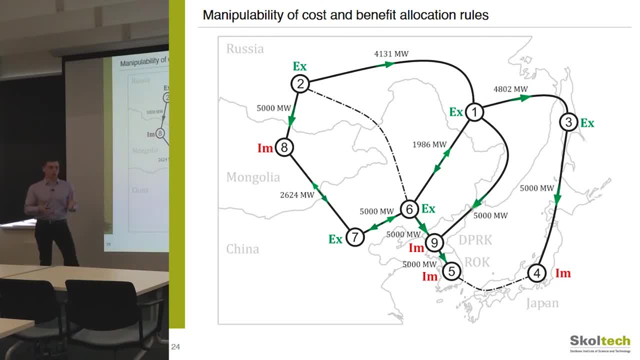 it may be more beneficial not to build so much capacity but to build less capacity, and to trade only with Russia, but at much better conditions. So, yeah, this is an interesting result that we published in the IEEE PowerTech conference Last summer. 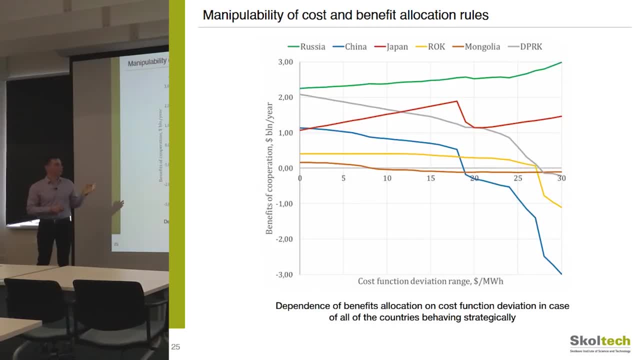 And also plots of what happens if all the countries behave strategically simultaneously in their own beneficial directions. And here the problem is that for only for Russia, the main power exporter, and for Japan, the main power importer, it is somehow beneficial to deviate. 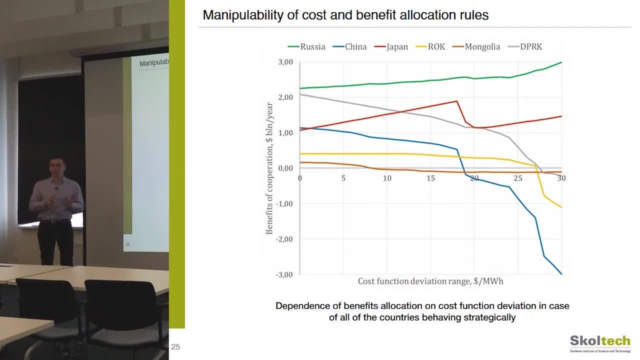 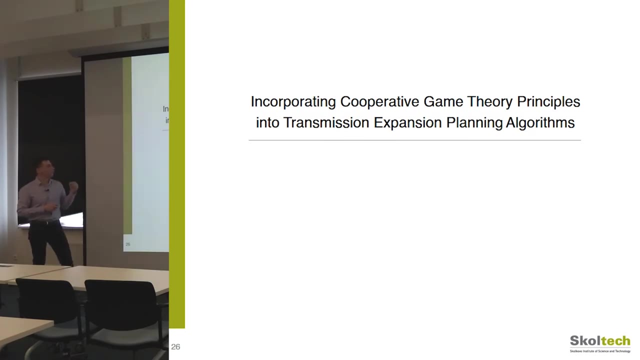 And for other countries in between positions, it is better not to cheat on their cost functions because they may get simply additional losses. Okay, And the last part of my talk for today, the recent results that we obtained. they are called incorporating cooperative game theory principles into the transmission expansion algorithms. 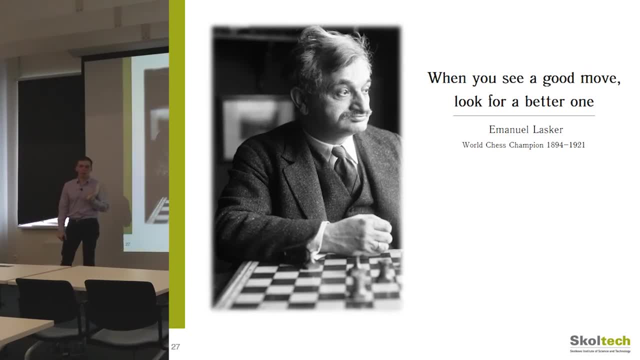 And I like to start this part of my talk with this famous quote by the second world chess champion, Dr Emanuel Lasker, who said: when you see a good move, look for a better one. And in terms of transmission, expansion planning. 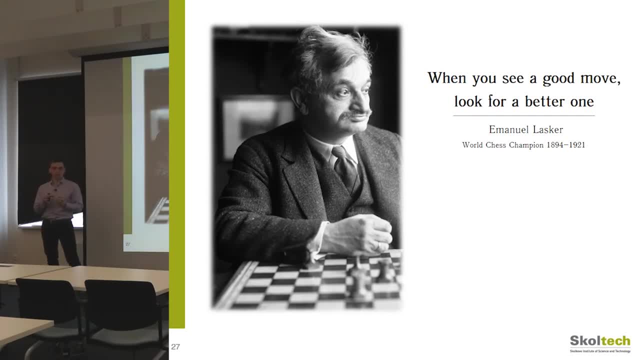 I think this could mean that if we see some optimal plan, maybe we should look for another plan that is better from some other points of view, maybe from cooperation points of view, And I will explain to you what I mean in a minute. 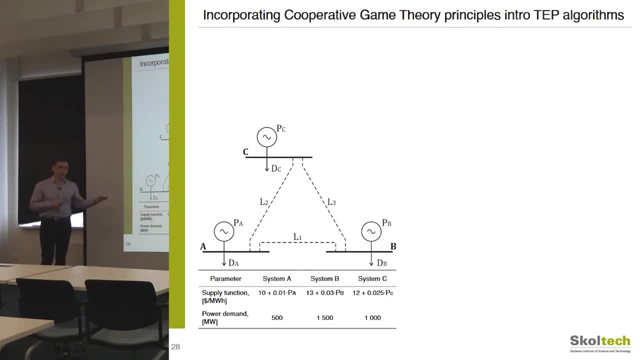 Last lecture I showed you already this example, the three power systems. Just to recall: system A has the lowest electricity cost function, system B is an expensive one and system C is in the middle conditions. And this is the minimization model. 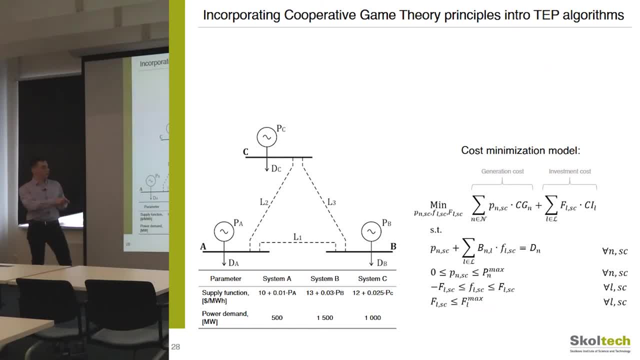 We minimize generation cost plus investment cost and we start launching this model for all possible scenarios, like no cooperation, the Grand Coalition. Please notice that all the lines are built up to 100 megawatts And for scenarios A, B. 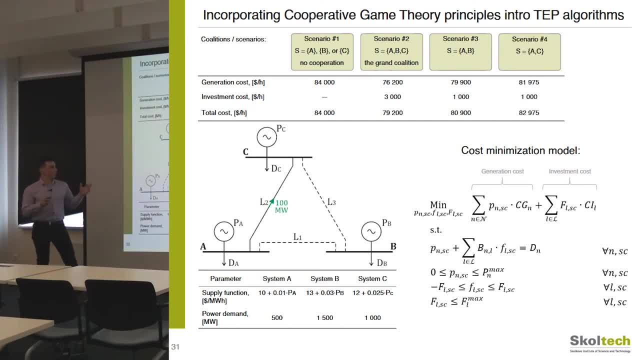 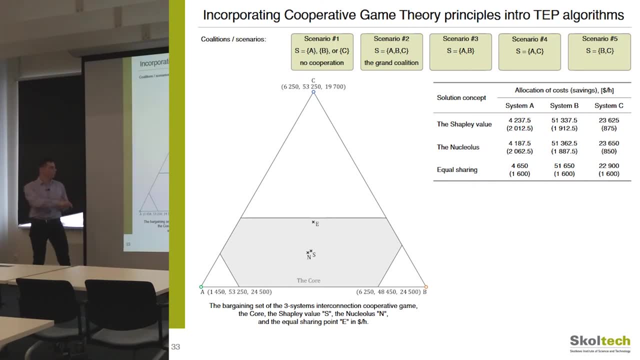 A, C and B, C. So we analyzed all possible scenarios and then we can calculate the Shapley value, the nucleolus, the equal sharing point. And you remember, this is the core of this, of the cooperation. 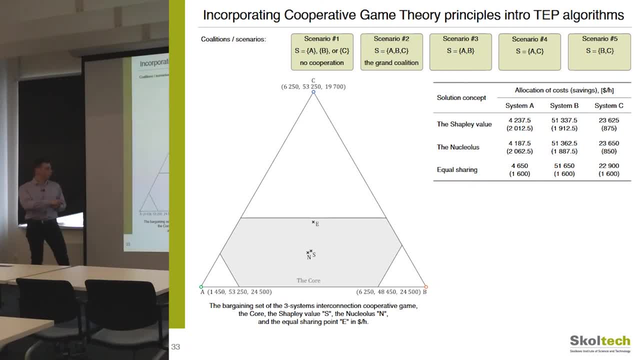 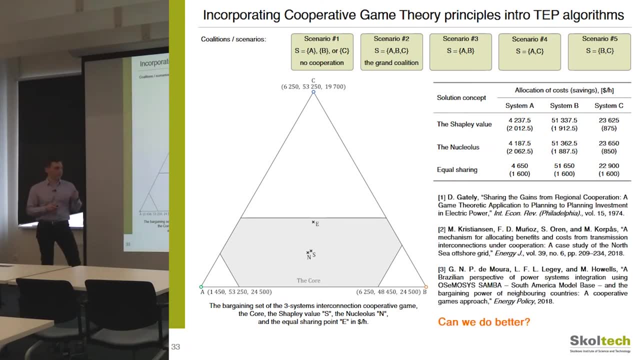 in this game- The equal sharing point, Shapley value and nucleolus, And I referred to some studies that did the same for the power systems, And the question here is: can we do better And can there be some problems with this approach? 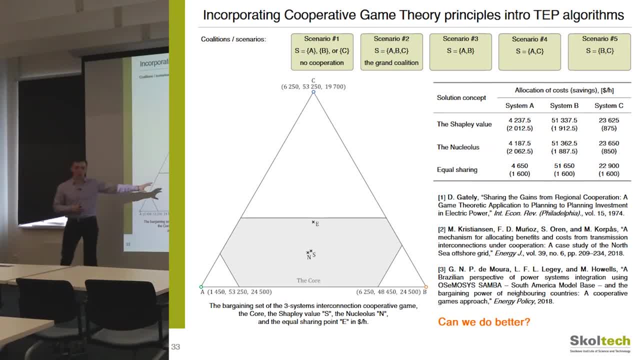 Well cooperative. game theory says that if the solution is in the core, then all the countries should be satisfied enough with the allocation. But in reality the situation may be different. There may be some mutual mistrust or some issues. Countries may have different expectations of how they should cooperate. 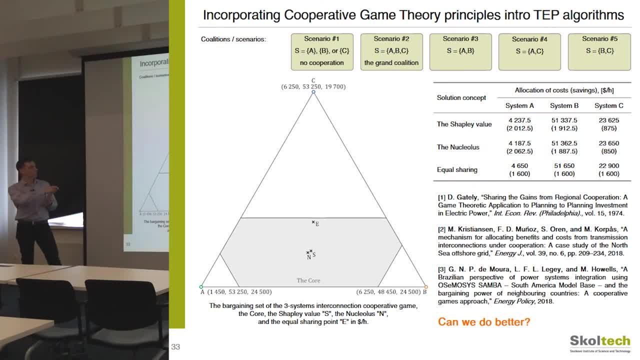 And you may notice that system C here is the less influential player. It is allocated not so much even by the Shapley value, And the core is rather distant from system C. So what if in reality system C says: I do not agree to cooperate on such conditions. 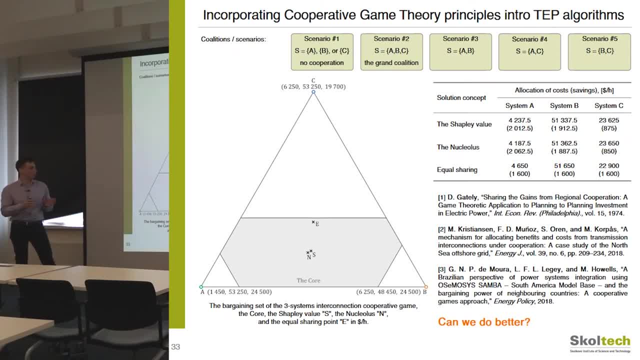 Yes, your techniques of allocation are good, but I just don't like that. I'm not such an influential player here And therefore the entire cooperation will be broken. So in order to deal with such cases, we suggested a reverse engineering approach. We would like to ask. 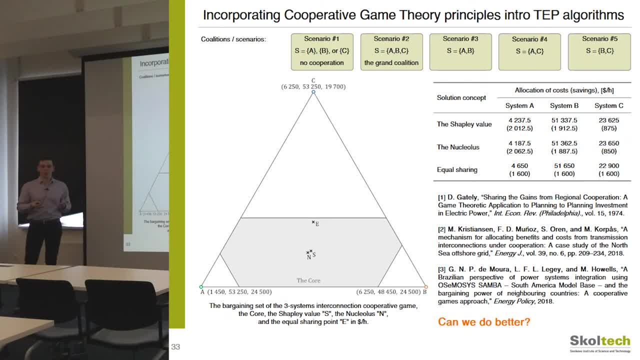 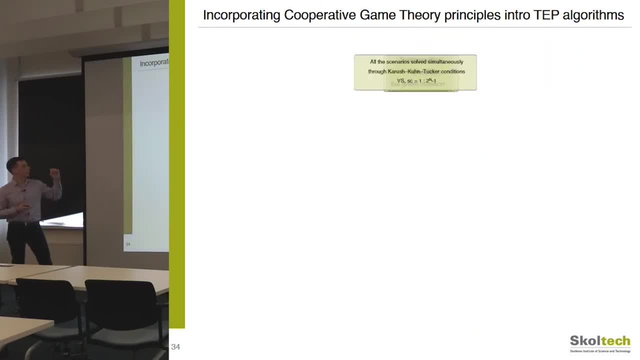 okay, what should be the transmission expansion plan in order to make the cooperation more stable. And here, by this animation, I want to show that we are trying to solve all possible scenarios of cooperation simultaneously in a single optimization model, And therefore we use Karush-Kuntaker conditions to represent each scenario. 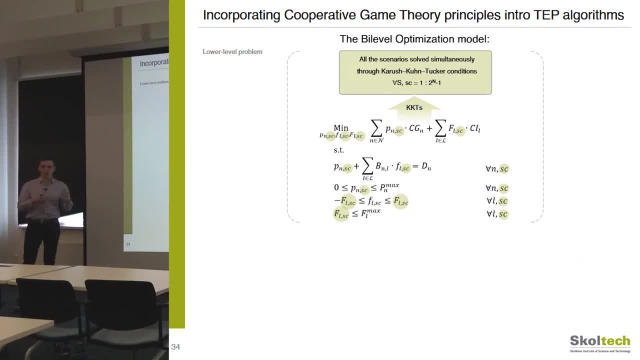 And by this way we formulate the lower level problem And if we solve it as it is, we will get the same scenarios, the same optimal scenarios that we already discussed. Therefore, we say that this lower level may be restricted by the upper level that we call cooperative game theory principles. 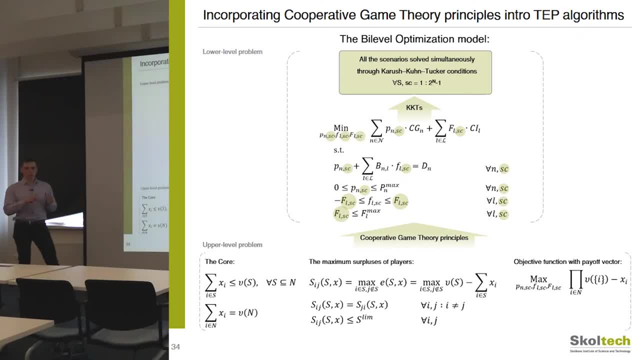 And here we may add any conditions into the bi-level optimization model, the core of the game, and also an interesting condition that we didn't discuss, haven't discussed yet. that is called the maximum surpluses of players. And the maximum surplus of player I over player J says what can get player I if not cooperating with player J? 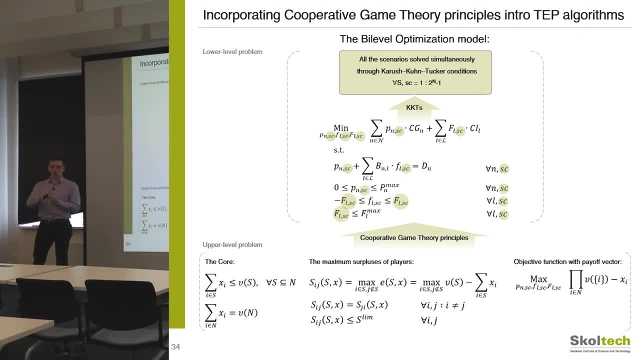 if joining some other coalition without player J. And sometimes this concept is called bilateral threats, because players may make threats against each other And here we say, okay, let's equalize all of these surpluses, Let's equalize all of these threats in the cooperative game. 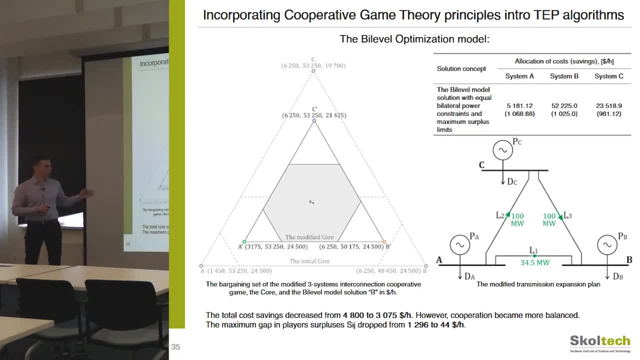 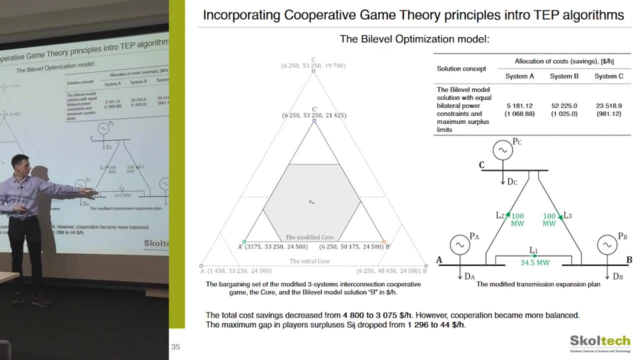 And we solve this bilateral model for the three power system case studies. And first look here. look what happens: Line one is not built up to 100 megawatts anymore, It is built to 35.1 megawatts. And now we look into the core. 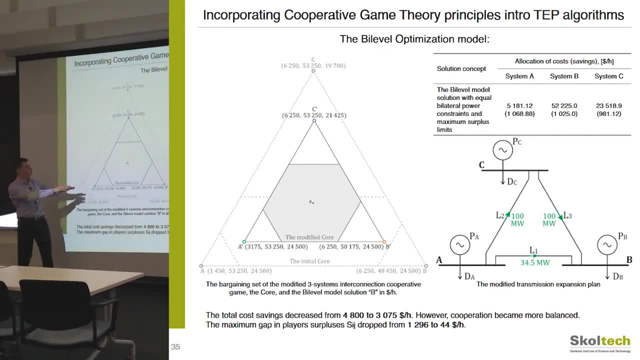 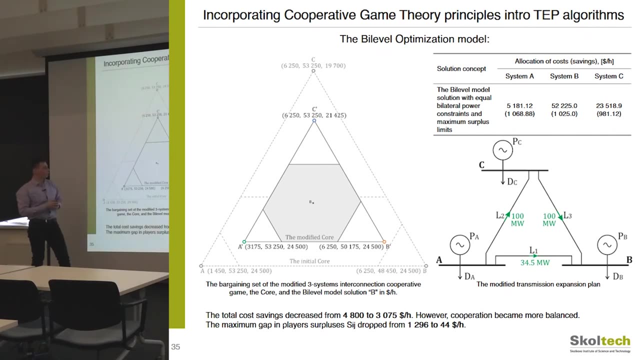 The entire bargaining set, the triangle ABC- it shrinks- decreased rather significantly. So this means that there are less savings of this cooperation, But the core, the structure of the game became more balanced And the solution is close to the equal sharing point. 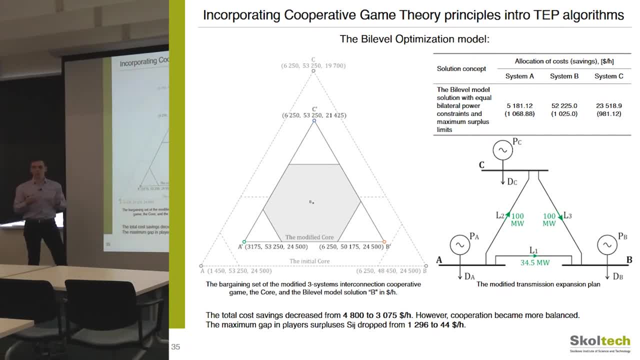 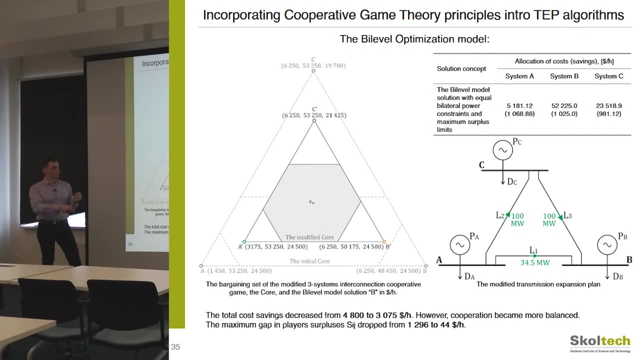 And this is an interesting idea that is close to the sanctions approach. We say that if you want countries to cooperate more equally, we shouldn't allow any optimal transmission expansion plan. We can restrict building of this line between the best power exporter and best power importer. 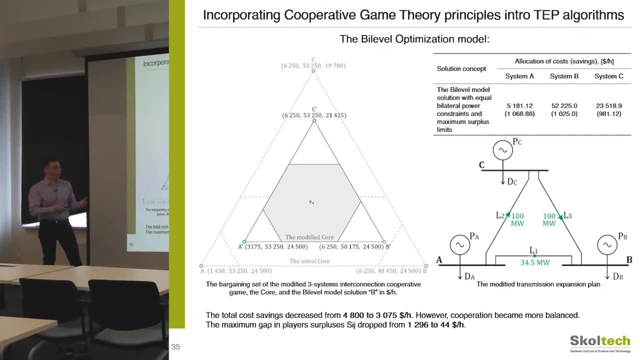 not allow it to build up to 100. And therefore we'll get suboptimal solution, but it will lead to a more balanced cooperation And I think this is an exciting idea. And the last case that I'm going to show you today. 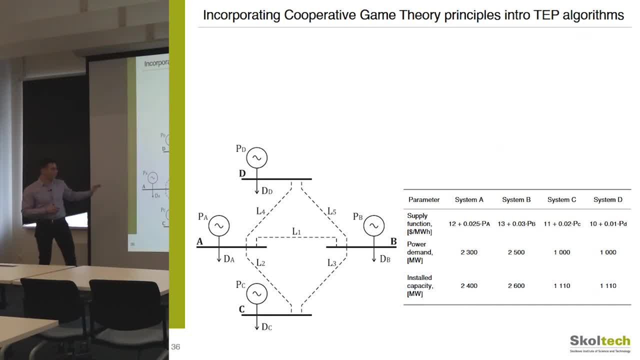 the same conditions but the four power systems, And here a bit different cost functions. System A and System B have the highest electricity cost And System C and D have rather low electricity cost And therefore they are going to, they're going to export power to A and B. 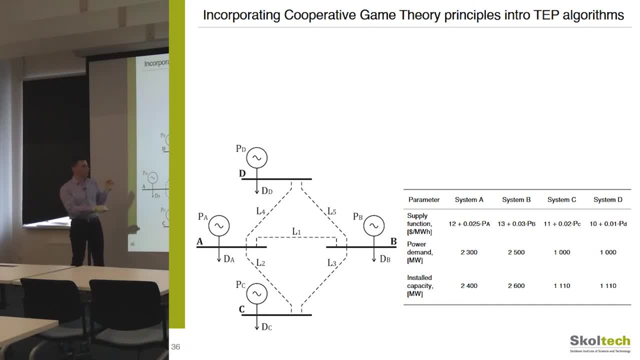 And also an interesting feature is that System B is a bit more expensive than System A. So if cooperation happens, System B should be the main power importer. And additional constraint here that systems C and D that are going to sell power- they do not have infinite power to sell. 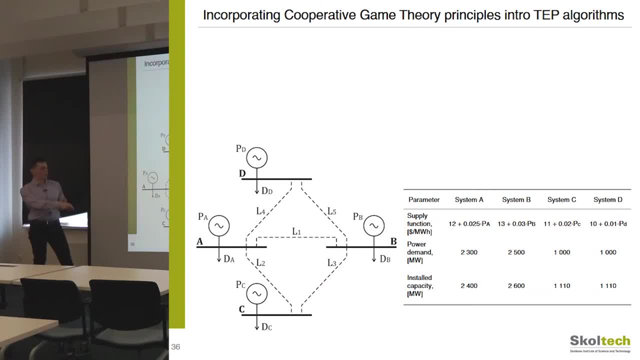 We say that they have only 110 megawatts each for for the export, So they cannot export infinite amount of power. And again we launched the optimization model, this scenario of no cooperation, the grant coalition and other scenarios for four. 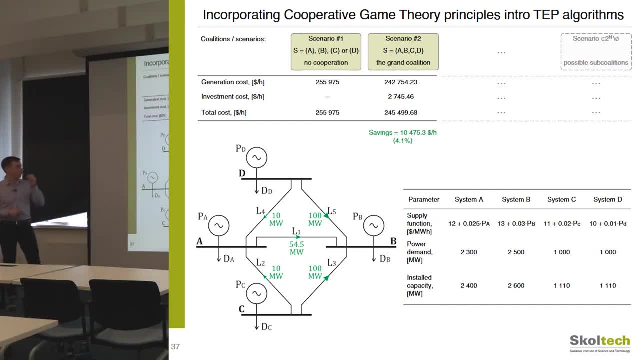 four systems. There will be 15 scenarios in total And we see that total savings reached $10,000 per hour, about 4.1% of savings, And this is the optimal power flows And we see that it makes sense. 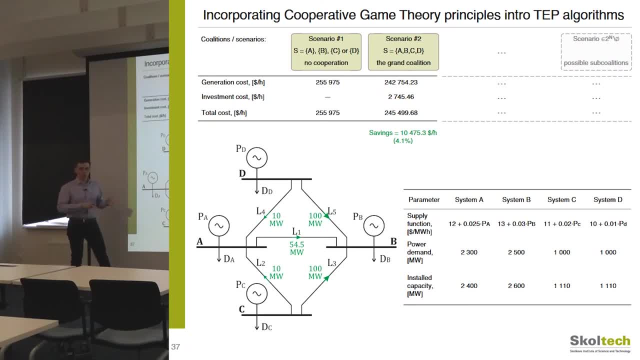 Lines five and three are built up to their maximum And all the cheapest power from systems C, C and D goes to the most expensive power system B, And this makes a lot of savings. But the question is, is this a good transmission expansion plan? 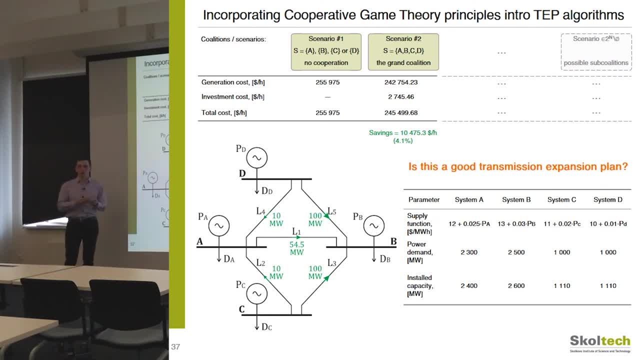 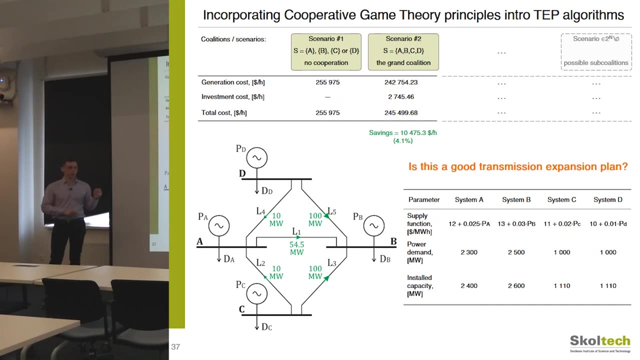 And indeed, in terms of costs, this is the best, the least cost transmission expansion plan. But I would tell you that, in terms of cooperation, this plan would be a. this plan would be a disaster, because I would argue that system A will be significantly underestimated in the grant coalition. 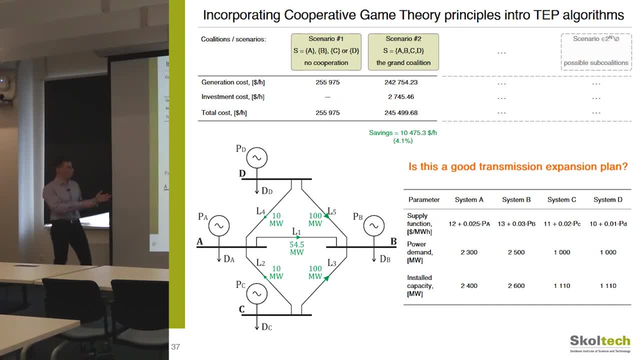 because in the grant coalition it brings almost no contribution. All the power systems would like to trade with power system B and get savings here, And only the remaining 10 megawatts flow to system A. But this doesn't mean that system A is a useless player, because in other 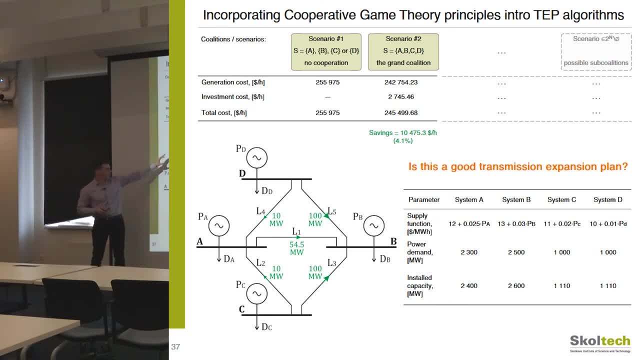 coalitions like AC, AD and ACD. system A is very important player And C and D would like to trade with system A and get savings together. So we see that there are two important players, A and B, but A is. 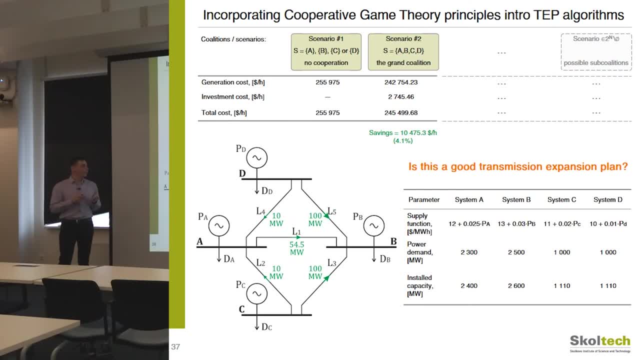 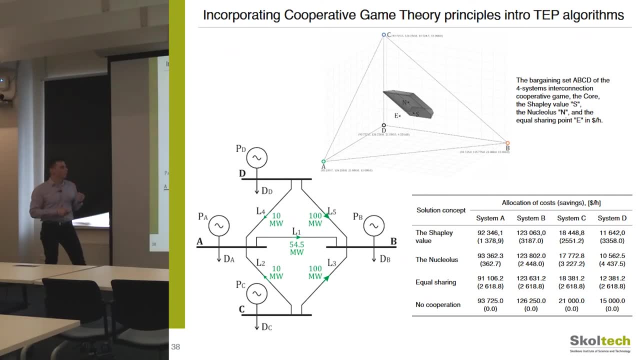 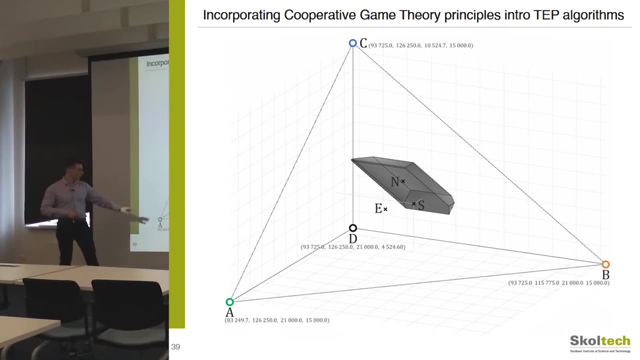 I would say depreciated in the cooperation. And we can plot the- yes, we can plot the solutions of this game and the core. Let's, let's zoom in and notice that, indeed, the core is significantly small in this cooperation and it is very distant from point A. 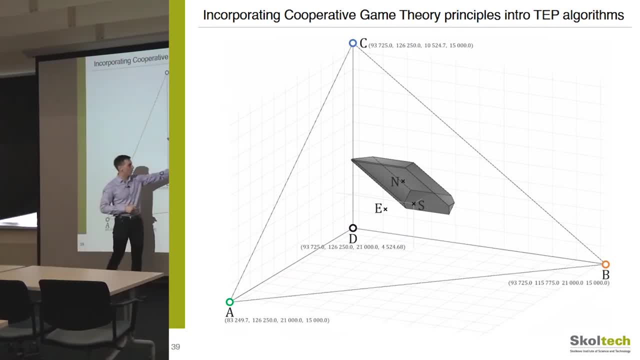 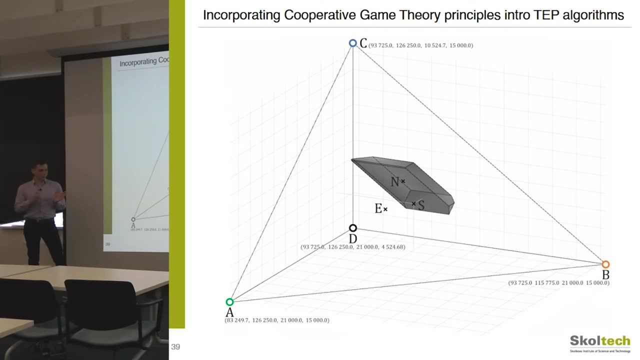 And it is so distant that I don't know. can you notice? but the Shapley value, it falls out of the core. So if someone of you would like to study this case, you will. you will find that the Shapley value is not in the core and some solution. 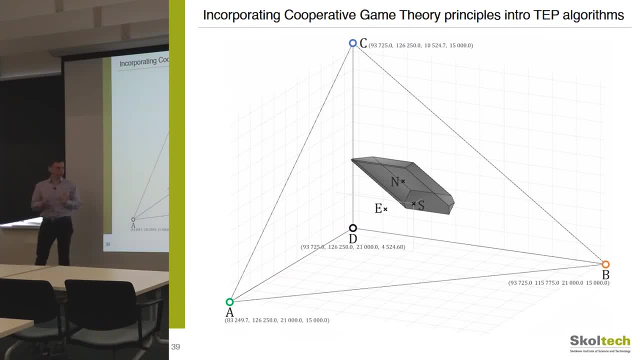 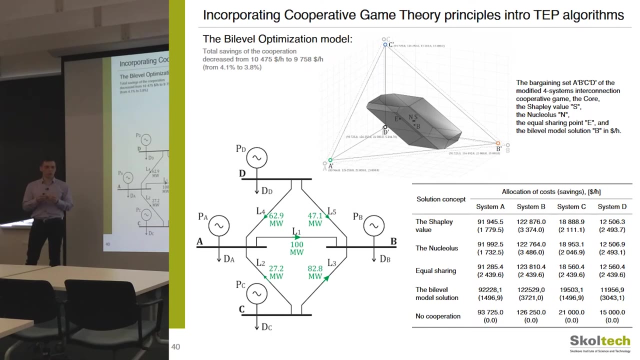 concepts will simply not work and the cooperation will be not stable. So we see that indeed, system A is underestimated in this coalition. And then we launched the my level optimization model, saying that systems should have equal bilateral threats, and we get suboptimal result. 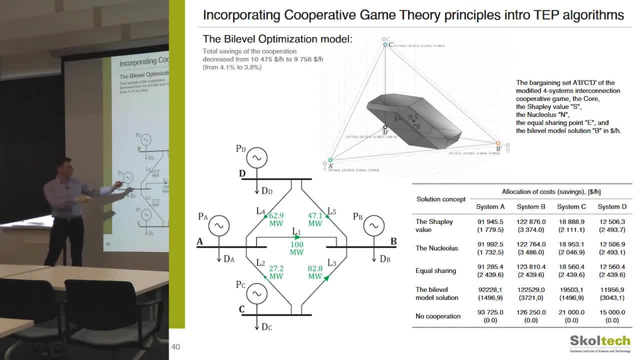 And first let's check what happens with the capacities. Lines five and three are not built up to their maximum anymore And instead these lines have much more capacity. And this suboptimal plan tells us: do not allow to trade so much power with system B. 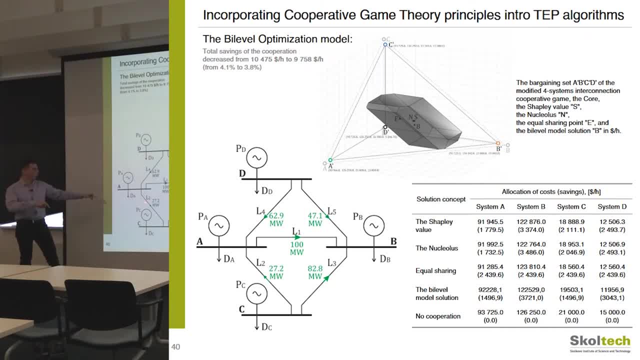 rather allow to the power to flow to A and then to B. So include the this uh expansion of this system more in the in the cooperation plan. This will lead to savings degrees from 4.1% to 3.8%. 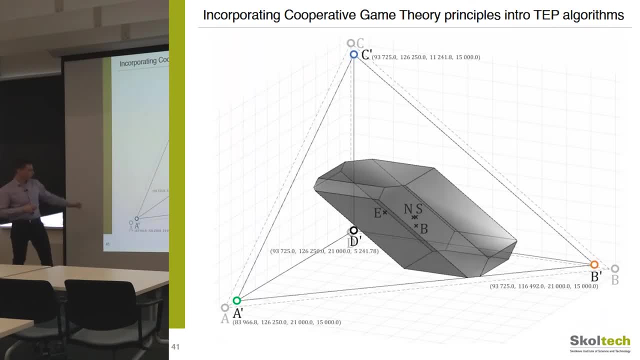 But let's take a look at the core. First, notice that here is a dashed tetrahedron and the solid tetrahedron and the new bargaining space, the new tetrahedron, this new pyramid. it shrinks a bit because there are less savings on the table. 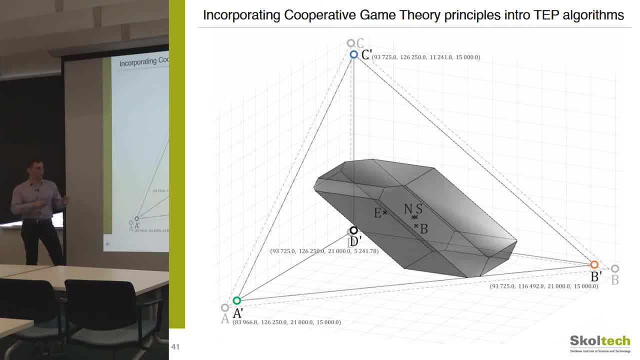 But the structure of the cooperative game changed dramatically. You may see that the core is significantly large here and all of the solution concepts, the Shapley value, the equal sharing point, they lie inside in the core. That means that this plan is much more stable for the power systems to. 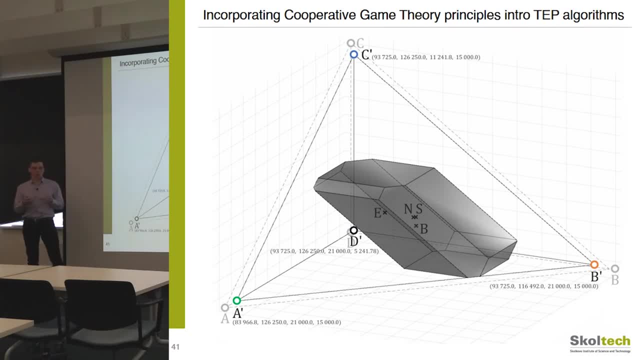 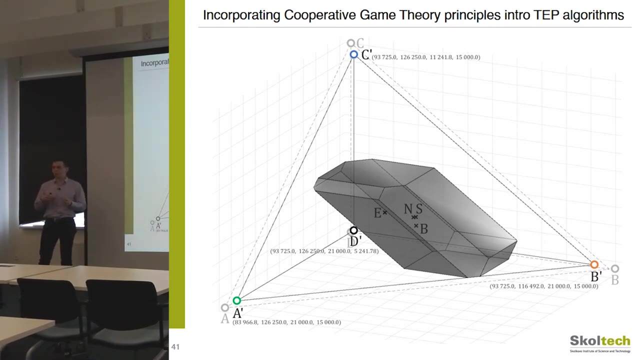 cooperate And I find this results amazing And I hope that you see how much space for research here is. when you implement game theory in some areas in power systems, how you can study the possible corporations. You may not even use game theory as an exposed analysis. 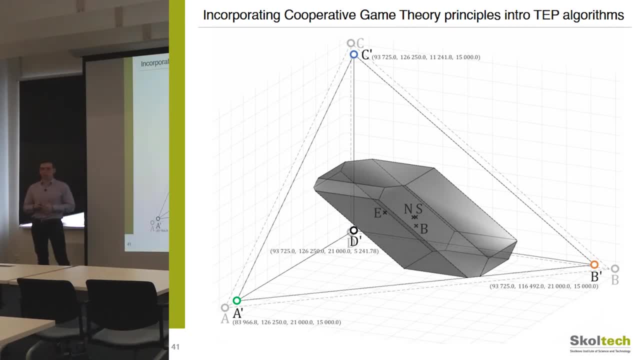 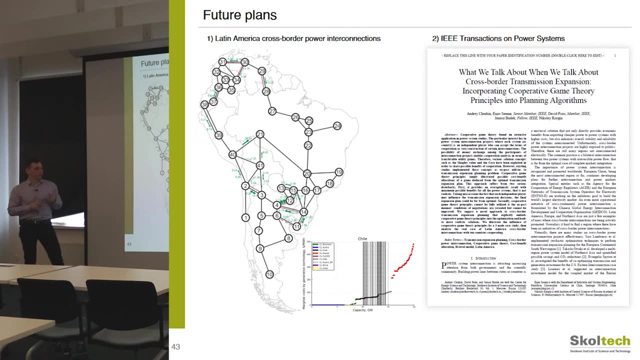 but you may embed these principles into your optimization model. And few words about future plans. We found reports of the Inter-American Development Bank with very interesting data for power systems in the South Latin America, For example. here I show just some data for Chile that we found. there are hundreds of. 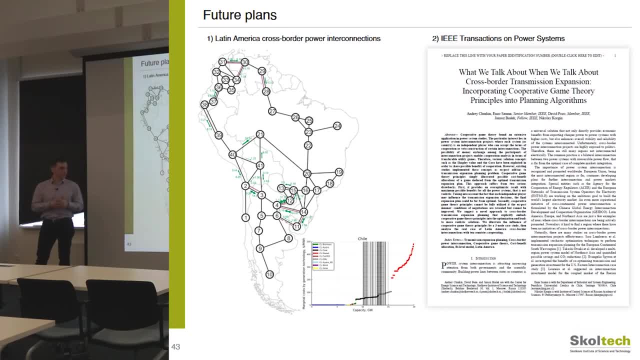 generations considered for each country, And we would like to repeat our analysis for this case study and also implement the bi-level optimization model with equal bilateral threats to see what should be the optimal plan and what should be the suboptimal plan, But that leads to a much more balanced cooperation. 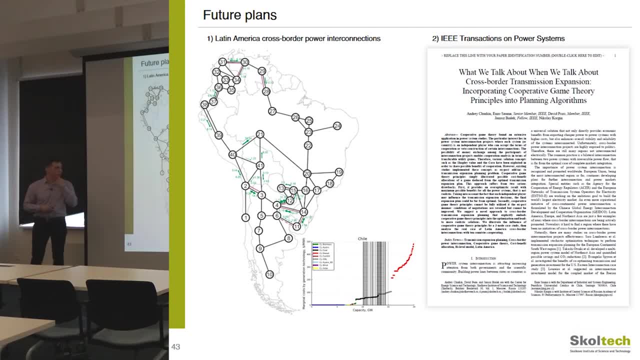 And we are still working on this case study. There are significant computational issues and we would like to write a paper to transactions of power systems. So far, this paper is called what we talk about when we talk about cross-border transmission: expansion planning. 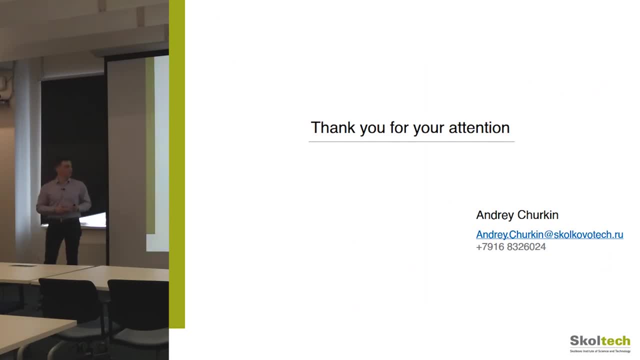 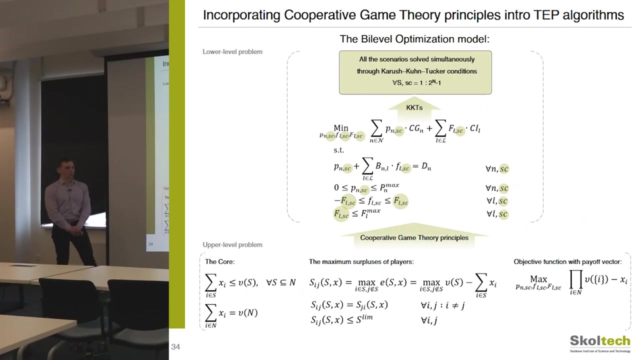 So I think I gave you a lot of insights and motivate you to use game theory in your own studies. So thank you for your attention. Any questions? Yes, please. Could you briefly comment about the computational complexity of the current? I cannot solve this yet for Asia with six players. 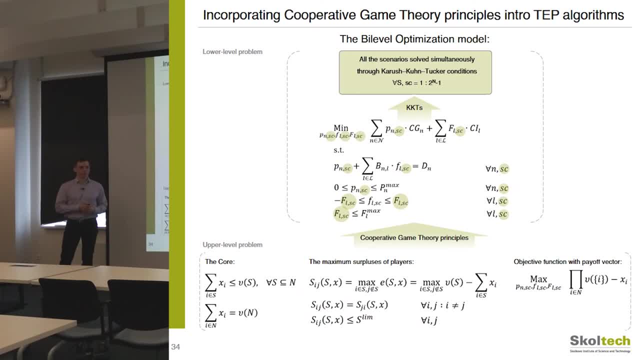 I solved it for four players, but for six players I cannot solve it. Yes, because you need to solve all of this bi-level problem simultaneously as a single optimization problem, And this means that you need to solve all of these scenarios together. 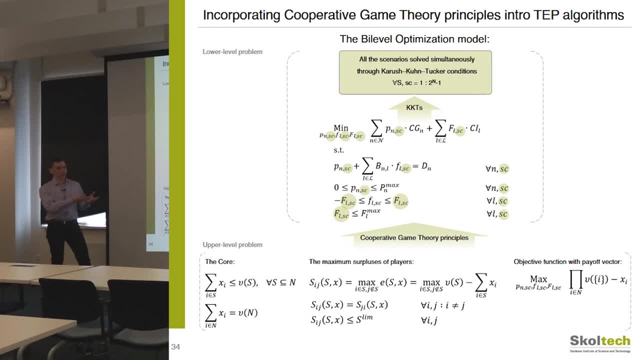 And you represent them as conditions. But then you get some complementarity constraints, multiplication constraints- You remember of the dual variables and certain conditions And you cannot just plug it in in Gurobi, for example, You need to modify it somehow, linearize with maybe big M approximation. 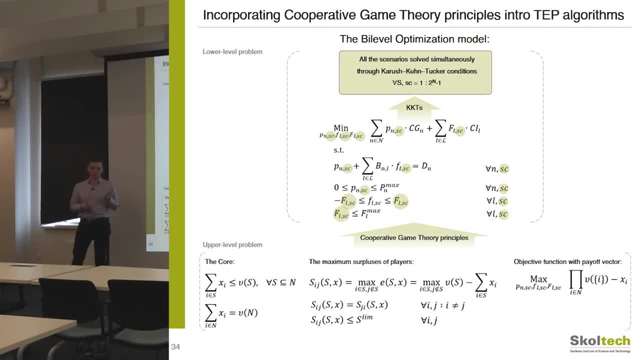 And if you and it becomes a mixed integer linear program, that is hard to solve For many binary variables And if you consider four power systems, you need to solve only 15 scenarios together And these constraints above of it. But if you plug in six players you get 63 of these problems together. 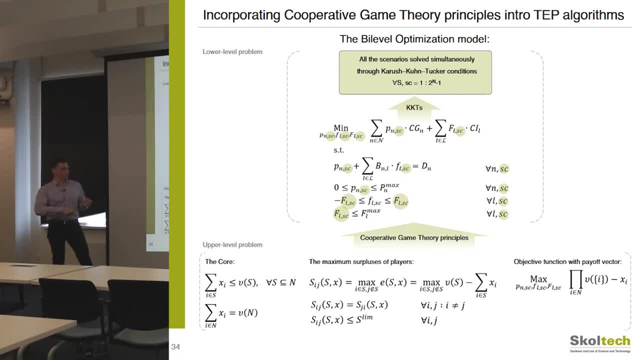 with a lot of binary variables, plus these constraints, And it simply doesn't work right now. We need to decompose it somehow. Yes, And for Latin America, for sure, it doesn't work right now. And there is another issue: sometimes, Maybe, you don't find a feasible solution. 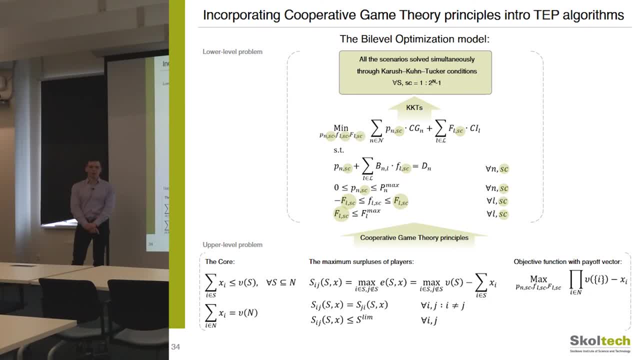 When you want to set this bilateral threat, it has to be equal for everyone. So I think that we have kind of this issue right. This is an unknown territory of research, because you don't know what you're looking for. Maybe there is no solution. 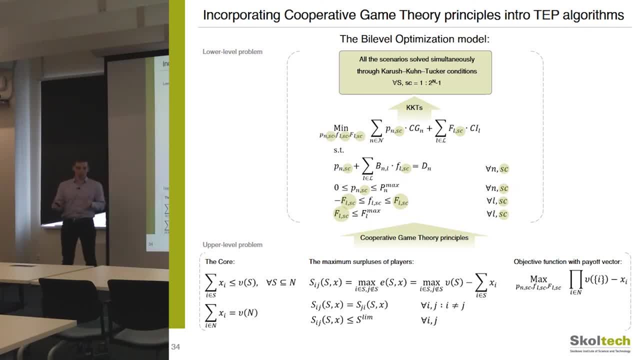 Because for some cases you say players should be equal, But equal may lead to no lines at all or some infeasible states, And I ran a solver one day for four days and it reached some level, But the gap was 2% or something. 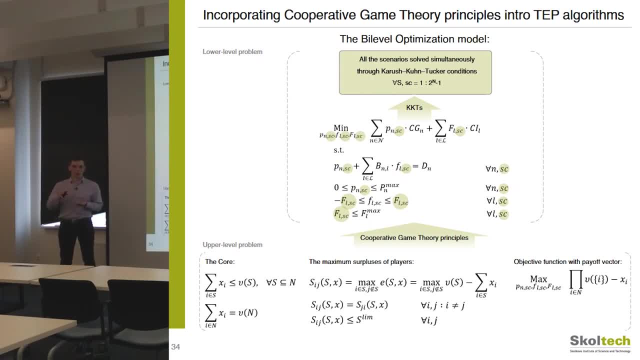 It's not good, I think. And then it was checking all possible combinations of binary variables, not moving for four days, So maybe it's infeasible, Maybe there are some better solutions. We don't know. It's a hard problem. 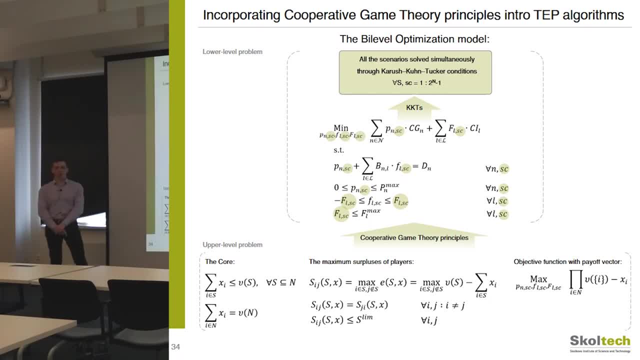 But for three- and four-player cases, fortunately we can get some insights, But in fact it will be very interesting and very valuable if we could calculate it. if I understand So, you were speaking about power flows distribution, right, But if you plan a path, 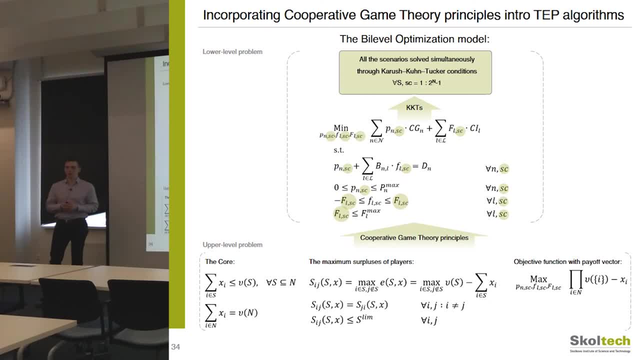 it means that you will be constructing some lines And if you're constructing them to have the optimal power flow and you construct them and then one player- which is very important, who is very important- decided to play a different game. you cannot change lines. 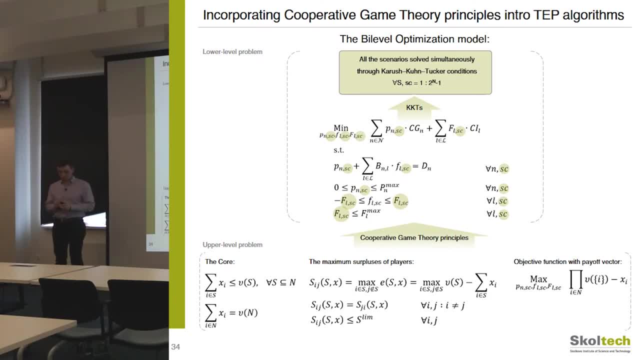 Yes, And if you spread the powers and weights of players more or less equally, it means that the disappear of one player or changing the rules by one player is not so dramatic. Is it right What you're talking about? you're talking about several stages games. 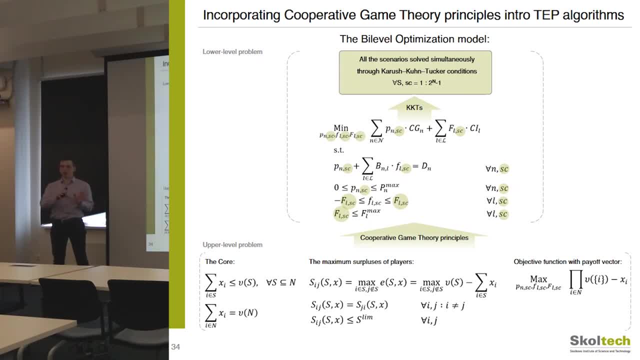 or maybe dynamic games, And here I considered only one snapshot, only one static snapshot of what happens before constructing the lines. So they sit and discuss what lines to build And it's hard to say what happens if you consider several stages. Then, as you say, first they decide what to build. 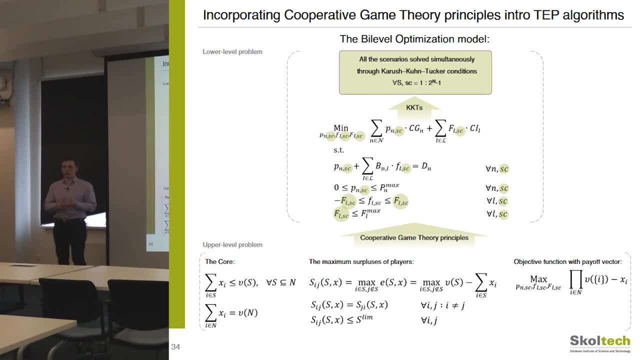 then they build and then they maybe leave collisions and do not trade energy. It's hard to say. I think there will be some complicated solutions. Isn't that the suboptimal solution where the weights are more? No, suboptimal is that? 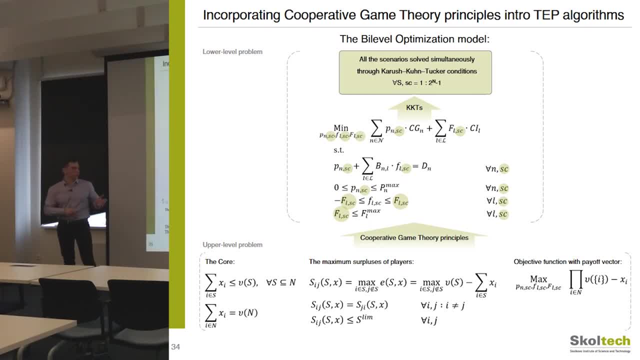 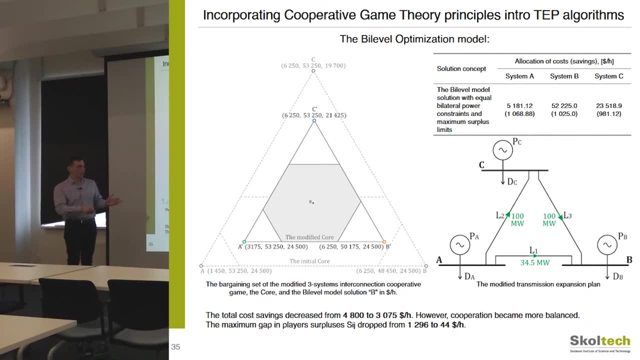 It's better. The optimal solution says: build here 100 megawatts. Suboptimal says: build here less power, because you need to make players more balanced in their influence on the game. This is the suboptimality that I'm talking about. 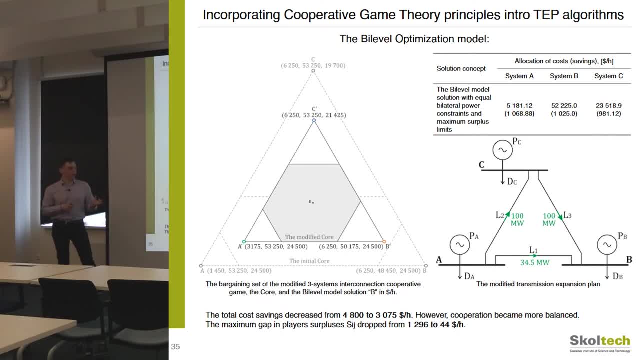 But this is just preliminary estimation of a project in a single snapshot. So yeah, last lecture I gave you some links about game theory And today I mentioned this TUG lab in MATLAB, So if you have any idea how to implement it, 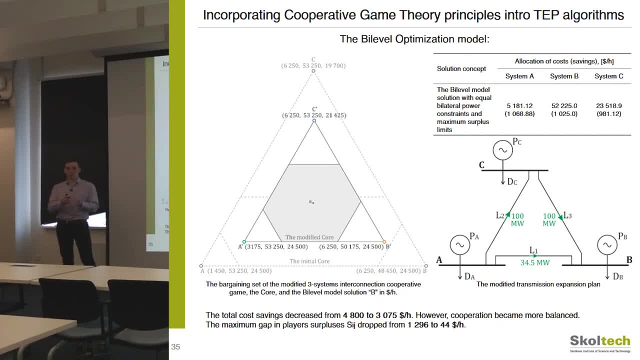 you can just watch it quickly or try experimenting: plotting your characteristics, giving your characteristic function to the MATLAB package and just analyzing what's going on in your cooperation. Is it good or not? Maybe this already will give you more ideas how to implement it. 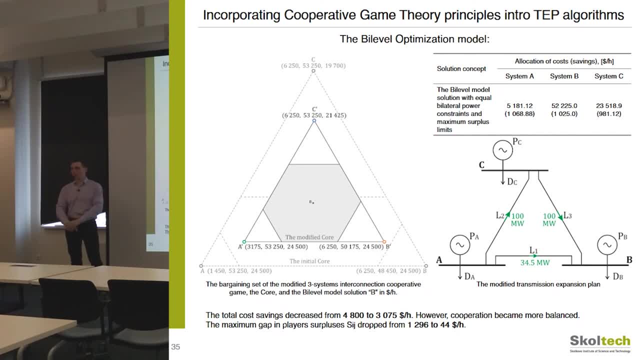 Okay, thank you. So I want to announce that next time we will have a seminar on the